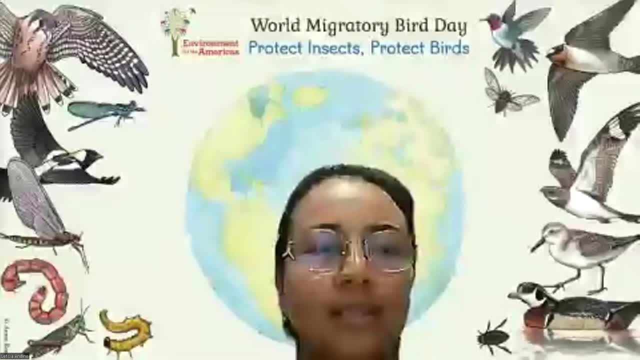 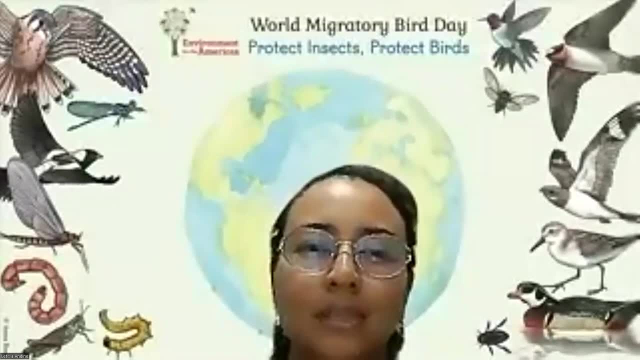 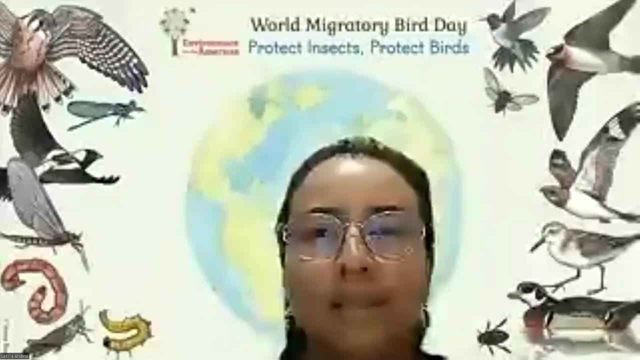 May you be very welcome to this third webinar. This is a series of trainings that we are developing for all the educators on the World Day of Migratory Birds. For those that don't know me, my name is Leticia Andino. I'm the coordinator of the campaign on the World Day of Migratory. 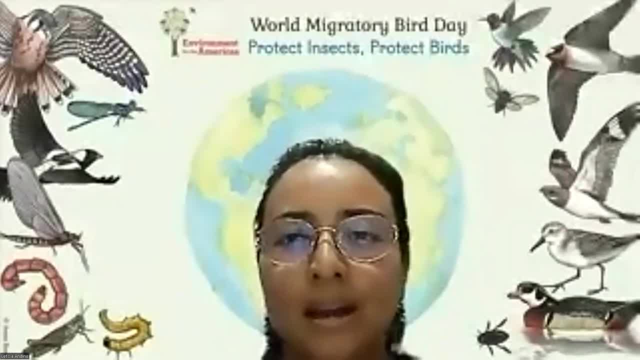 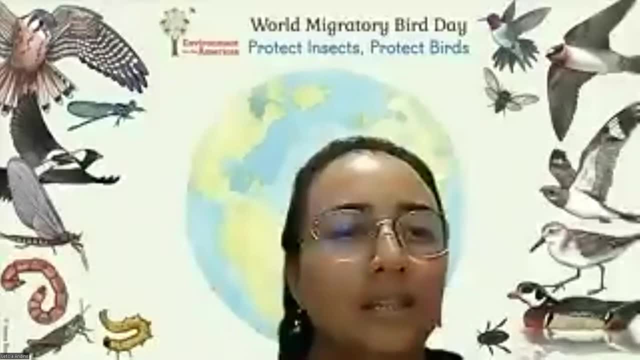 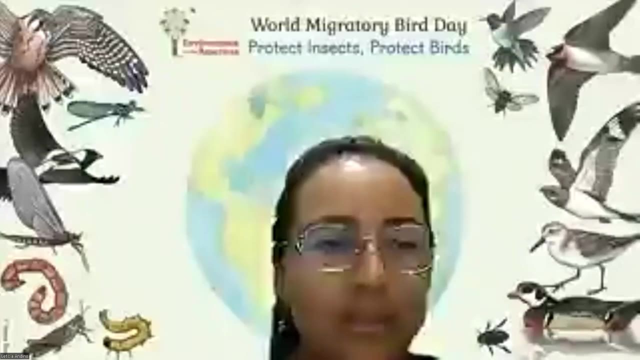 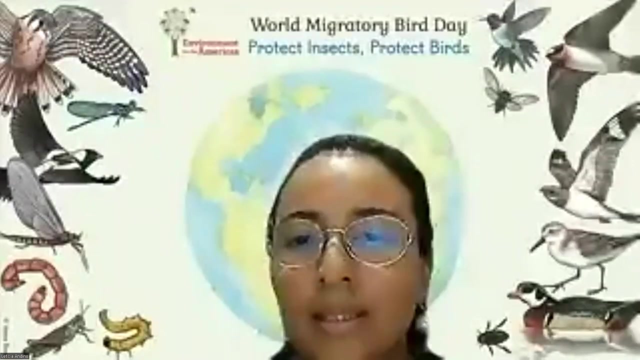 Birds for Central America. So welcome to everybody in Central America, South America, Mexico, the Caribbean, North America and from the different places that are joining today. I am going to present today in my screen what we're going to see today. We're going to get to. 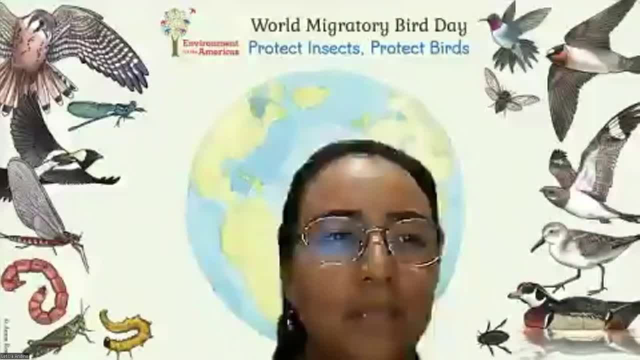 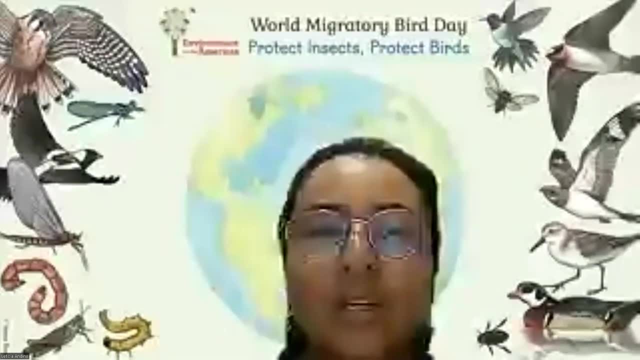 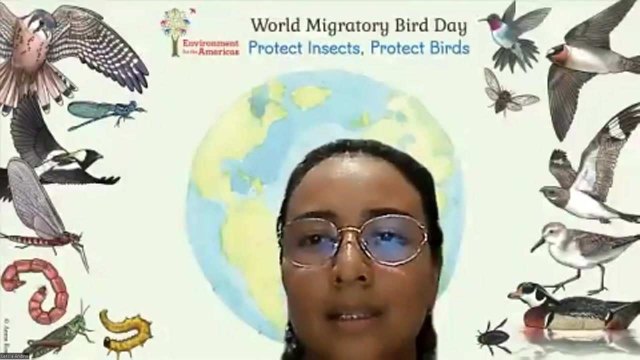 the group of insects and also the group of birds. In our group we also have other coordinators from other areas and other regions: Laura Babula from the Caribbean, Miguel Mata, who is the general coordinator of the campaign and also coordinator of South America. And 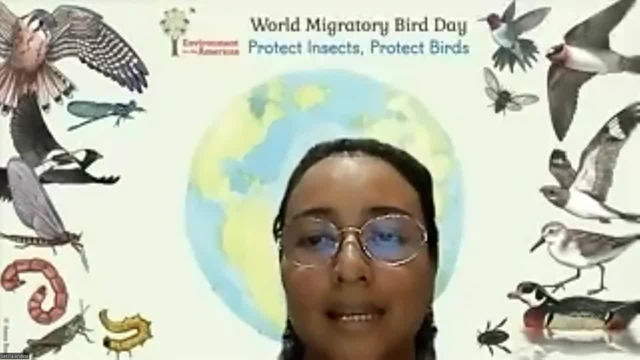 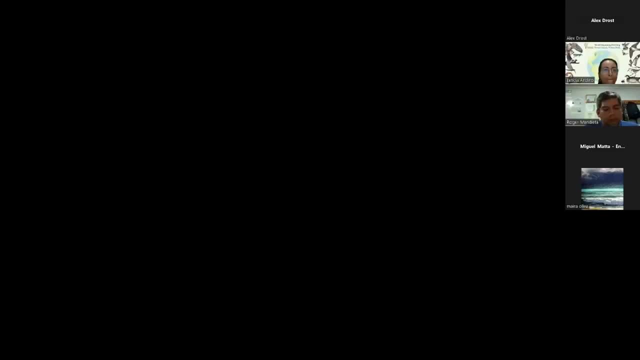 I'm going to present today in my screen what we're going to see today. We're going to get to the group of insects and also the group of birds. We're going to get to the group of birds. If he is curious about the group of birds, they're go-to guides. We also have these wonderful computers. 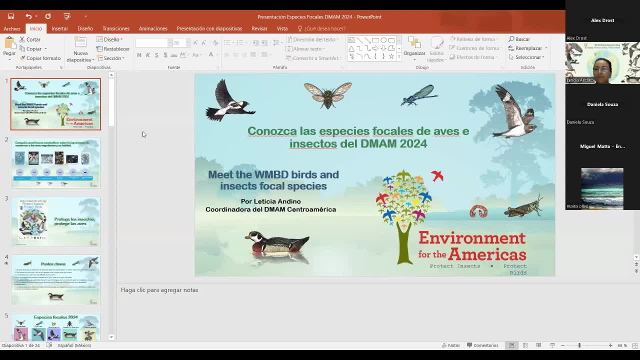 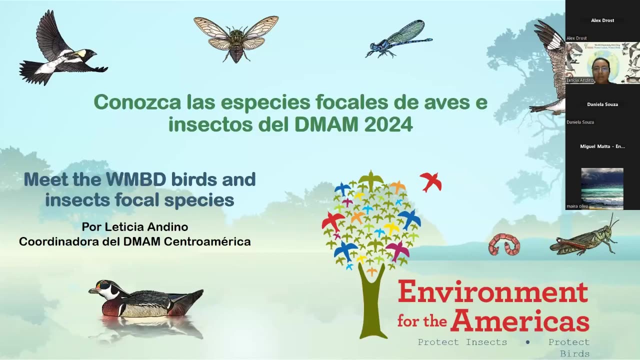 here, and these are the ones that we have here everybody. We also have a littleuestestly moved into the area of the world in this virtualeoolныхnet classify of birds. So let's get started. Here we go, But knowing a little bit more about the focal species that have been selected for the campaign for the World Day on Migratory Birds, and also the insect. 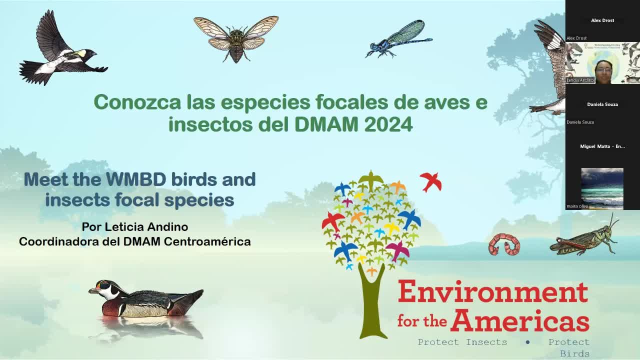 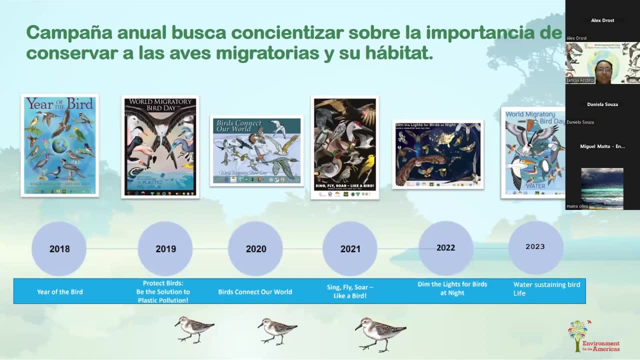 As you know, this annual campaign is trying to raise awareness, the importance of maintaining the habitats of migratory birds, So each year we take on a topic, a different topic, for conservation. So here's some of the topics that we have taken on since 2018 to 2023. 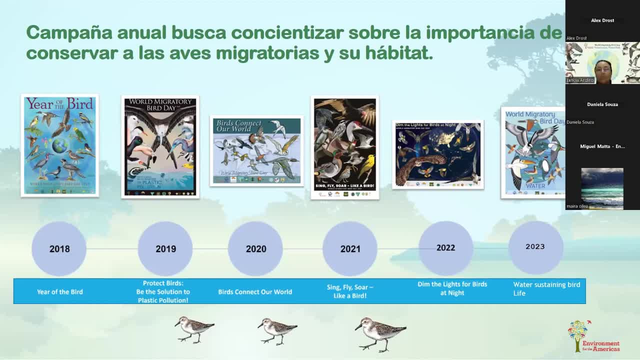 For example, the campaign on passion for plastics. This was about becoming aware and sensitive to how plastics, especially plastics of one youth, is affecting many birds, Specifically those in the water In 2022,. we also saw a topic that was quite interesting, which is the light pollution and how this affects the migration of birds, specifically those that migrate during the night. 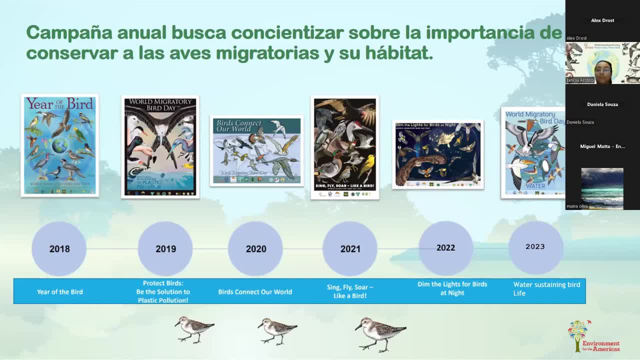 And also how it affects those resident birds during their reproductive stage During 2023,. we saw- Please test The topic of water- water that is vital to birds- And we also saw some of the actions that we could take on from our homes, our community, our jobs, so that we could actually provide a more amicable environment for birds. 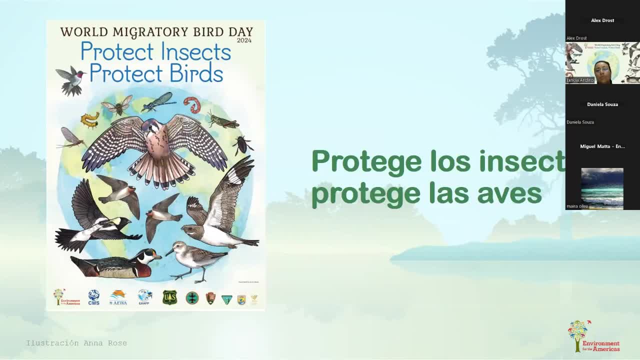 Now we go to 2024, which is to protect the insects, to protect the birds. As you can see here in this poster that we designed, there's the different species that have been selected as representatives of the different regions, And some of you participated in some of the formats that were filled out to select these birds. 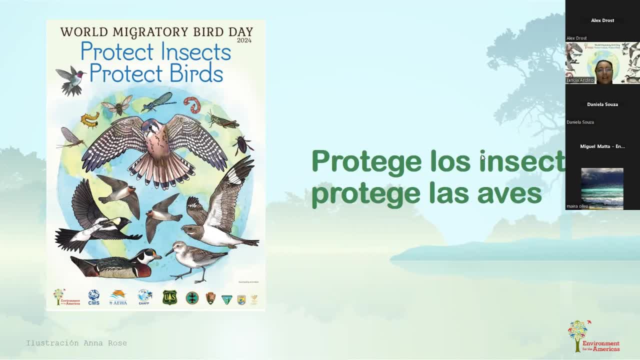 And these were selected as representatives of the different regions of the hemisphere. Amongst them also are insect species, So we're going to start seeing each and every one of them in this presentation. This illustration is thanks to our artist, Anna Rose, who is our artist of 2024.. 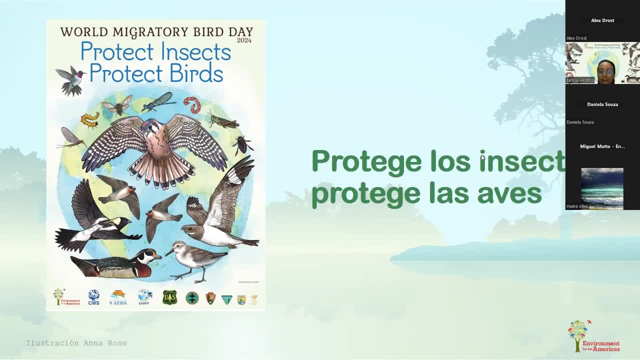 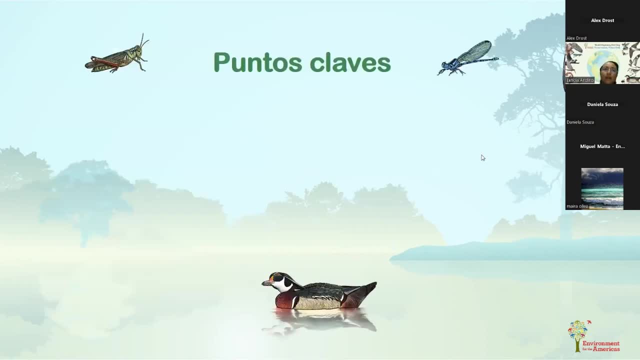 She was big in her ability and experience to depict birds and insects. All right, to give you more about the context of why this topic was selected, I am going to show you a little bit of the context of why this topic was selected. I am going to show you a little bit of the context of why this topic was selected. 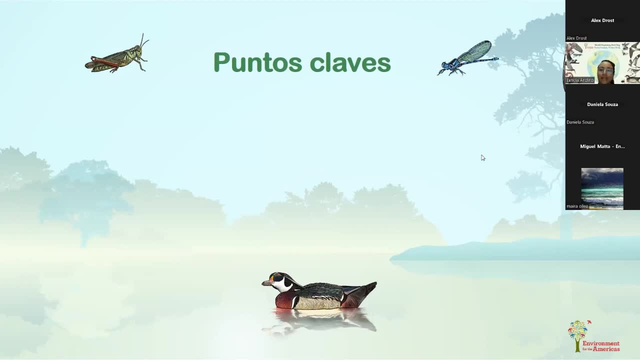 I am going to show you some of the points that relate to this group of insects and birds. One of the key points is that many birds that are feeding of insects are disappearing at the same time in the same places. Many of the scientists think that, since the population of insects is decreasing, 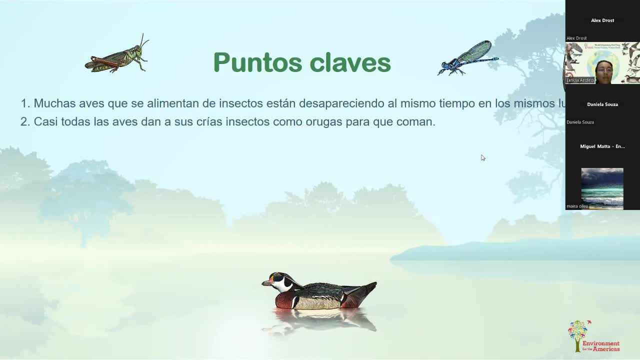 many of the scientists think that since the population of insects is decreasing, then the population of birds that consume insects is also decreasing, then the population of birds that consume insects is also decreasing. Number two: Almost all of the birds give insects for food when they reproduce. 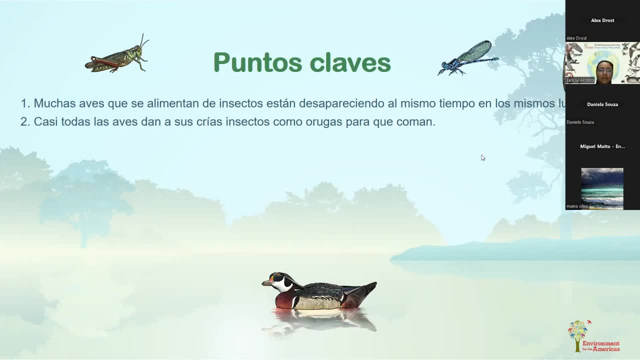 Almost all of the birds give insects for food when they reproduce. So the hatchlings in my summer batch will give the insects of mismo with a few упraus. But one thing we understand is that the insects have a lot of mu? desses been repeatedly taken out by the dragonflies. 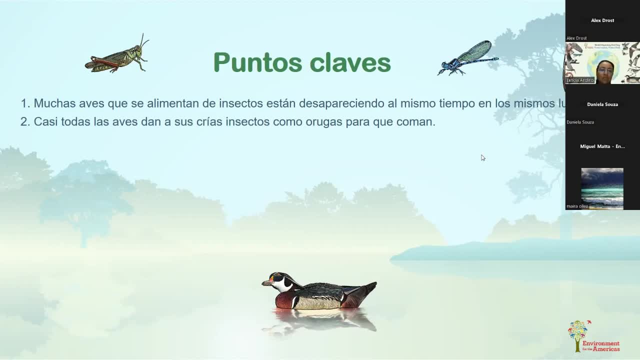 The dragon: it is removed due to ins clue stabs via the bulla. The dragon: it is removed due to ins clue stabs via the bulla, which, at the first phase of their growth, have a hard time to consume the seeds. then they're given. 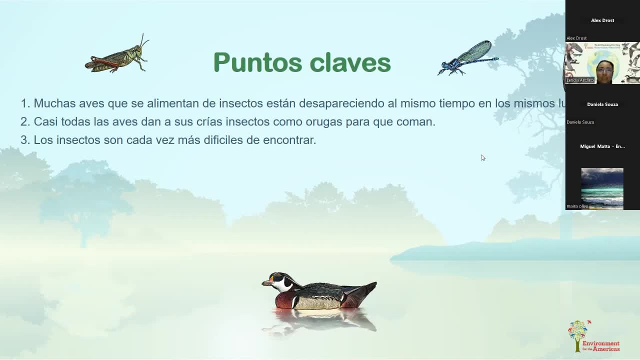 insects by their, by the birds, the parent birds. so the insects become each and every year harder to find. this is due mainly to human activity: the change of the growth of agricultural frontiers, the use of pesticides, other changes in the soil. also, migratory birds capture. 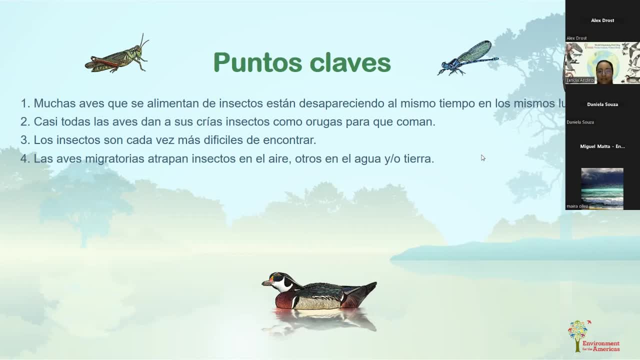 some insects while flying, others in the soil, others in the water. so finding them in many of these environments, in these spaces that usually these insects are, have been polluted or, as I told you before they are being used to, there's been use of pesticides, so this decreases. 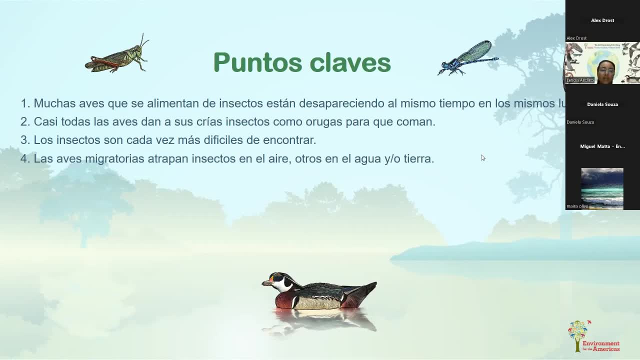 the population of insects in different places, places that birds tend to go or have the knowledge to go to find food. point number six, number five sorry- is the generalized use of pesticides. pesticides, they are used to control the insects that are considered pests in the crops. 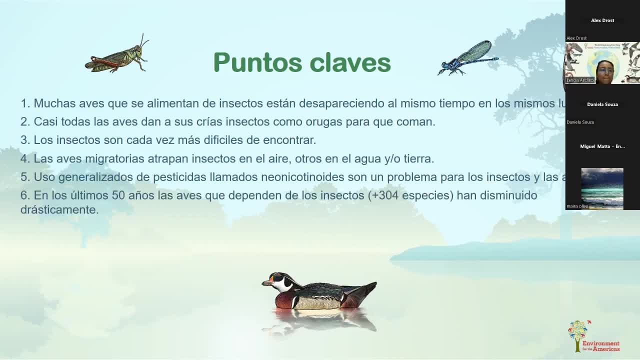 and therefore the birds are called neonicotinoids. these are the types of pesticides that are used and that are a problem for insects and birds also. in the last fifty years, the birds that depend on insects, which is about three hundred and four species- these have diminished drastically. 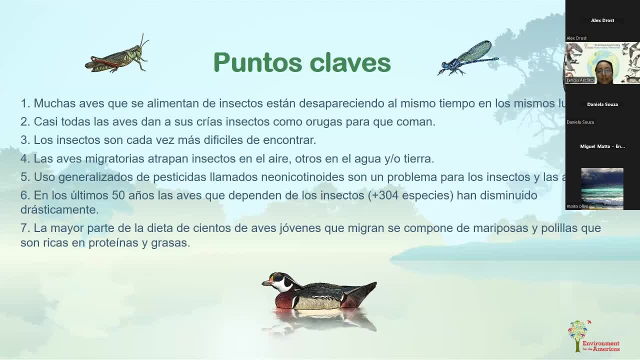 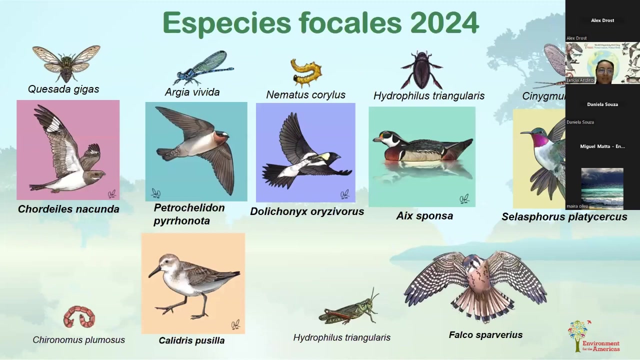 in the last few years, and also most of the diet of young birds that are migrating is by mainly butterflies and moths. these are a great source of protein and other nutrients that are needed. these are the focal species that we picked in our research in two thousand twenty four. 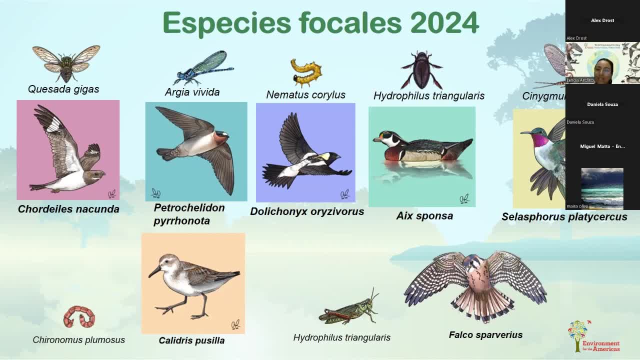 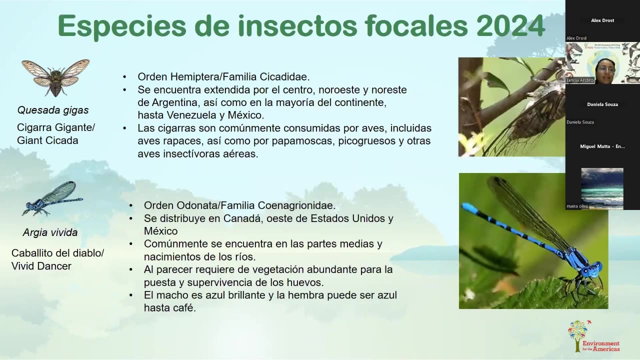 these are seven species of insects and seven species of birds. we're seeing the generalities of each and every one of them, so we're going to start with the group of the insects. as you can see, this in this slide is the giant cicada here in El Salvador. 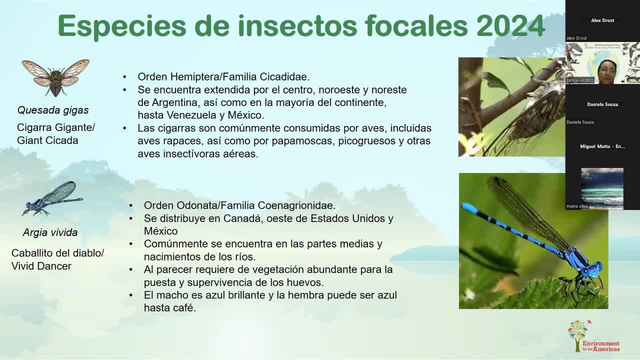 we call it chicharra. I don't know how it is called in other countries, but this one is mainly found in the center, northwest and northeast of Argentina, as well as in most of the continent, the hemisphere, and it can come all the way to Venezuela and Mexico. 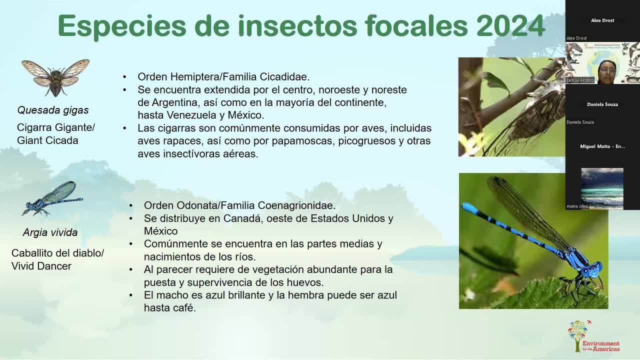 the giant cicada are usually consumed by birds, but also they are usually consumed by birds, but also they are also some predator birds, as well as other species. the chant of the giant cicada could reach up to 96 decibels. this is their call for reproductive. 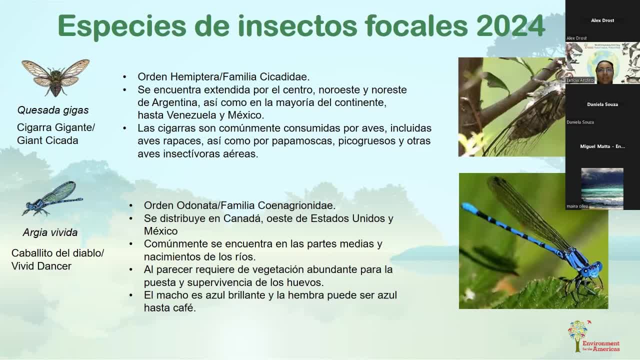 activity, and it's also been compared in its strength to fans, motors and other type of their. larvas can remain for years under the earth, feeding off the roots of plants, and it's quite important food for different species of birds, just like the ones I just mentioned. 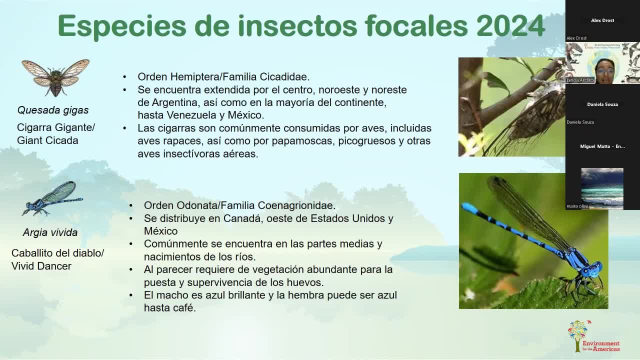 the other species of birds that you can see is called caballito del diablo. it's from the odonata order. it's distributed in Canada called vivid dancer, and also you can see it in the United States and in Mexico. you can see it in the 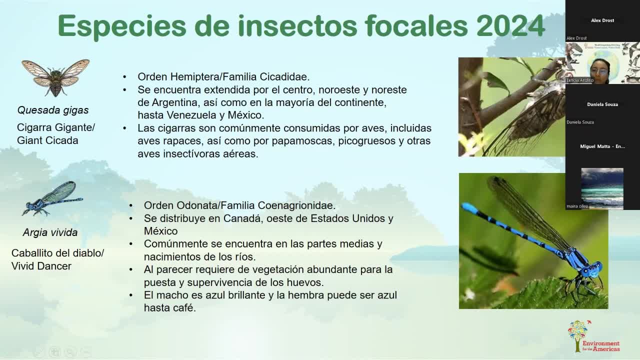 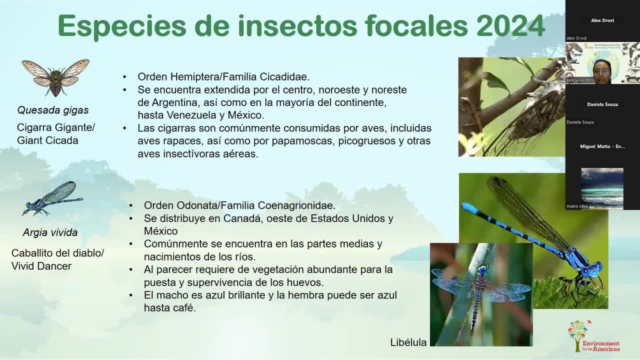 really clear, it's very clear and it's it's very yeah, yeah, Cassandra States, m p, pac, per p, ef, ah, eh o. let's move on right here to next. and The specialists are convinced that without the presence of these types of insects, and as well as dragonflies, we would be in dire need. 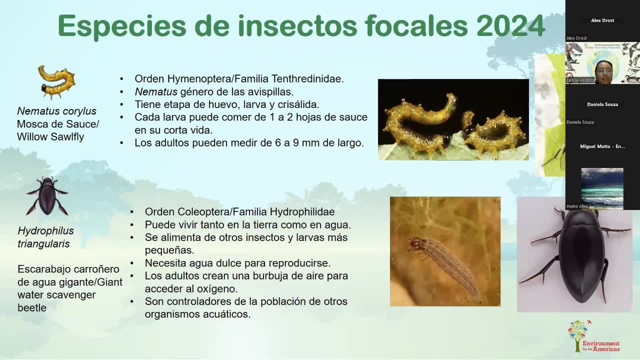 Basically even the plagues of a smaller insects that transmit some very contagious diseases. So, going to the next, we have the willow sawfly And, from the order that the gender is nematus, Each larva could eat. Each larva could eat. 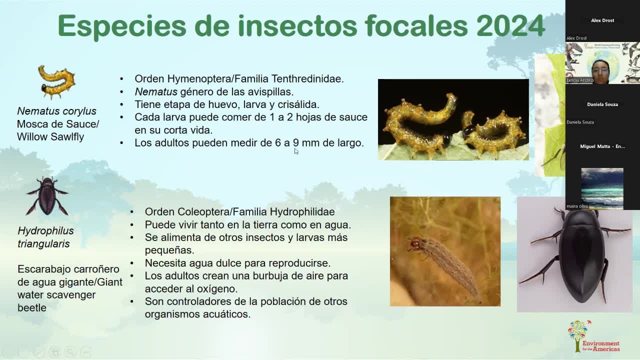 From one to two Weeping willows leaves during their lifetimes, As you can see here in the picture. this is how they grow when they have fully grown. So we have a picture of the larvae and then a fully grown picture. 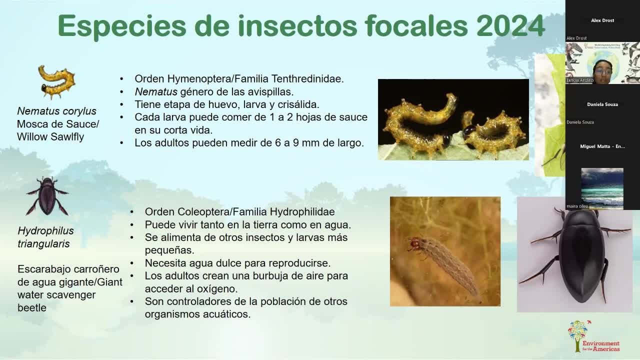 And what we have below is the giant water scavenger beetle. They can live both in land and water, Feeds of insects and smaller larvae And needs fresh water to reproduce. The adults create a sort of air bubble underneath their wings. This is they become hardened and they could be used while they're underneath the water. 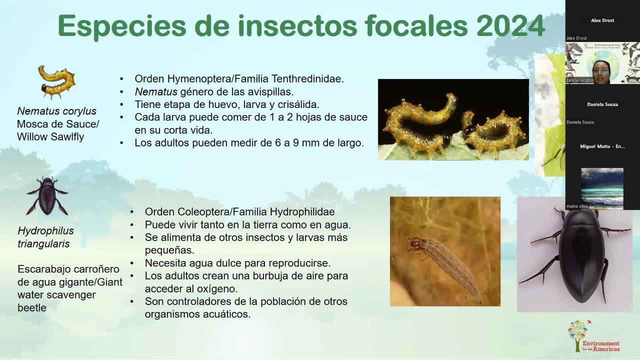 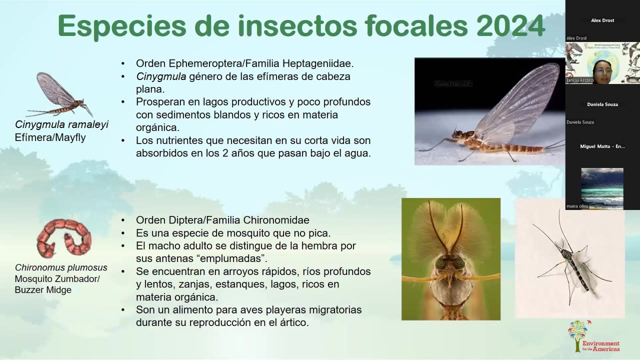 And those become connected to this bubble of air And that is how they can take on the oxygen from the air. These are very important because they control the population of other water organisms that have been traced along with them. Other of the focal species that we have is called the mayfly. 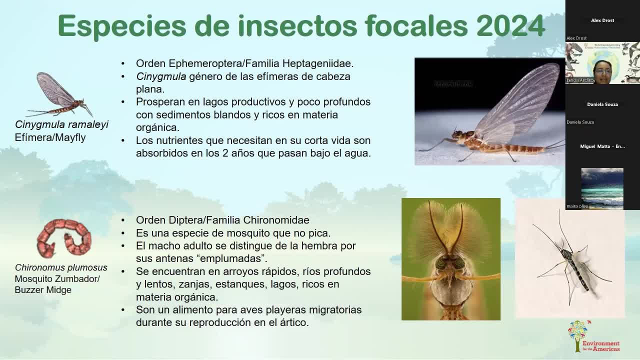 It comes from the Ephemeroptera order. The mayflies reproduce in shallow lakes that have very much of an organic matter at the bottom. This is the kind of nutrients that they need during their short lives And when they emerge from the water. 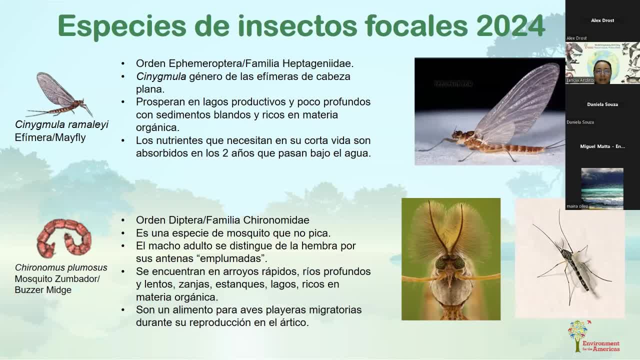 They emerge in great groups, large groups, And this is how they become into very important foods for birds such as the hummingbirds. On the other hand, you also see below what is called the vassal midge. This is a type of mosquito. 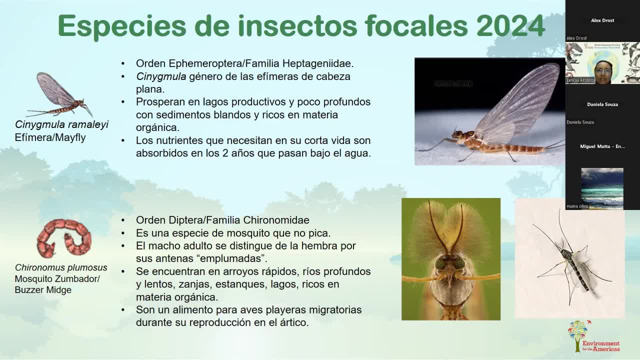 This is a type of mosquito. This is a type of mosquito that doesn't bite, but that it is found in areas of the Northern Hemisphere. The larvae of this species is a very important part of the food chain. Once they, the mosquitoes, emerge from the water. they are also known as blind mosquitoes. 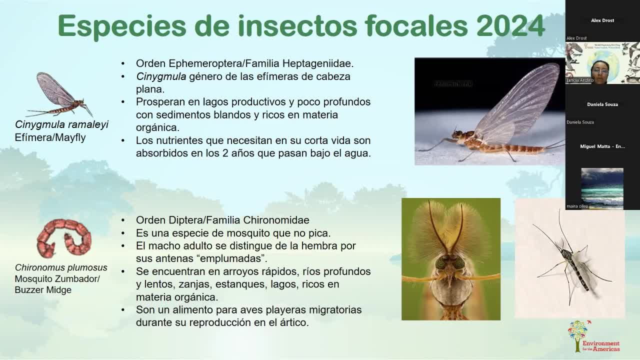 They sort of look like a mosquito, but they don't bite humans. You can see in the picture the male. the adult male is distinguished from the female, given the sort of feather antenna that they hold, These sort of antennas. they look like feathers. 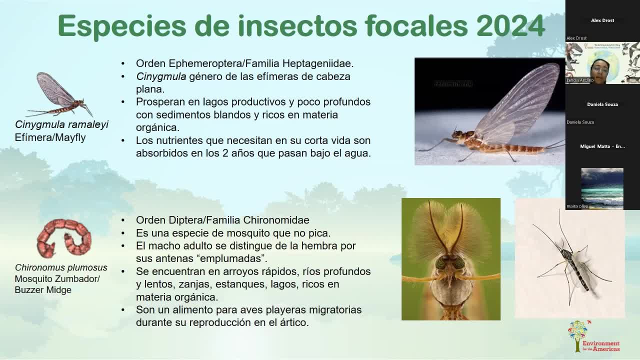 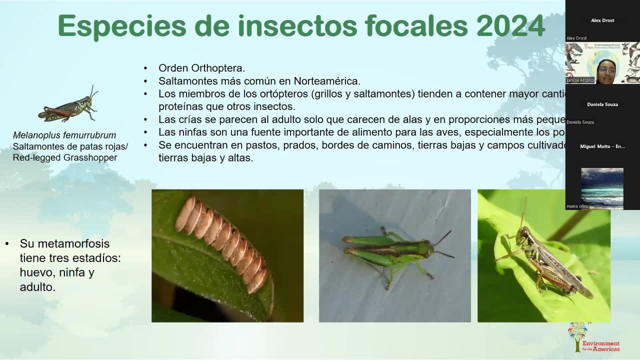 You can find them in ponds, ditches, lakes, anything that is rich of organic matter, And they are very important during the reproduction of migratory birds in the Arctic. Another species that we have as a focal species is the red-legged grasshopper, also from the Orthoptera order. 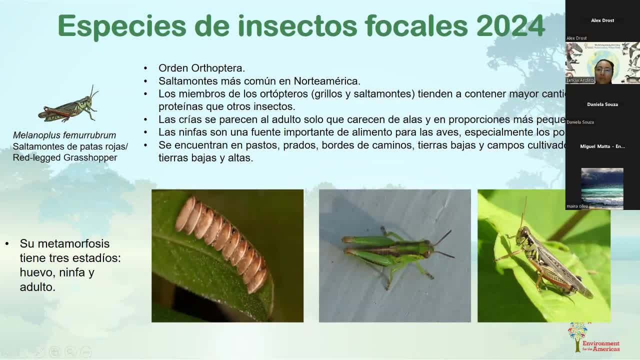 This is one of the most common grasshoppers in North America. It's the same order as crickets and grasshoppers that are the most predominant and hold a great amount of protein compared to other insects. When they're in their youngest stage, they look like the adult, but they're just smaller. 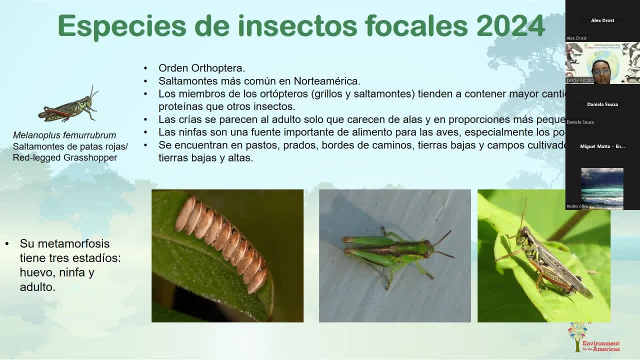 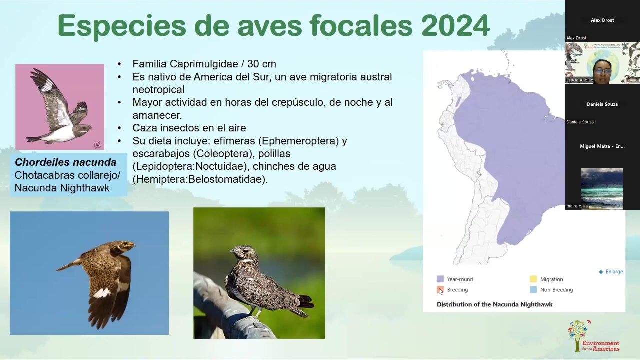 The nymphs are rare. The nymphs are quite important for the chicks in their young phase of growth, And they are also found in grassy areas, lowlands and some crops. So these are all the species that we have called focal species. 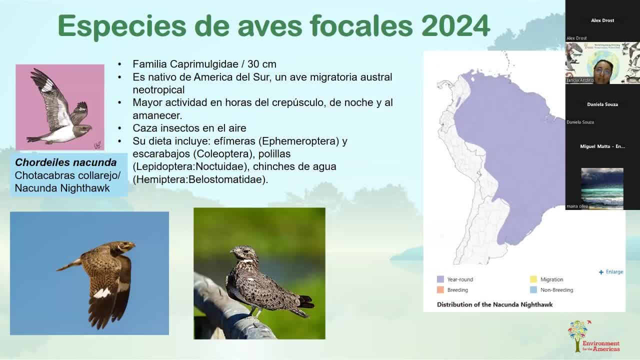 Now let's go to the focal bird species. Let's go first with the Naconda nighthawk. We have many names in El Salvador for this species. It's native from South America. It's an austral migratory bird, neotropical. 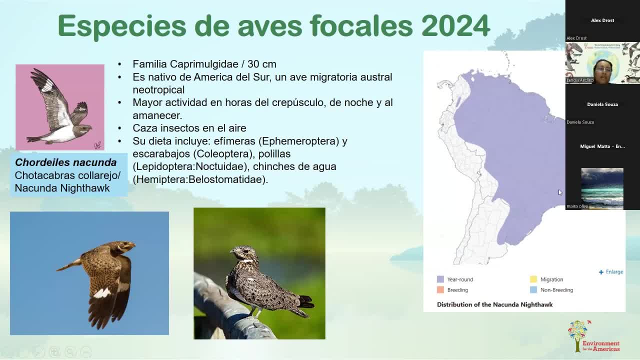 And you can see it here in its distribution. To the right you can see the map which is the distribution area. It has activity during the sunset, at night, early morning. As you can see, its distribution can come all the way from Colombia, Venezuela, Trinidad and Tobago. 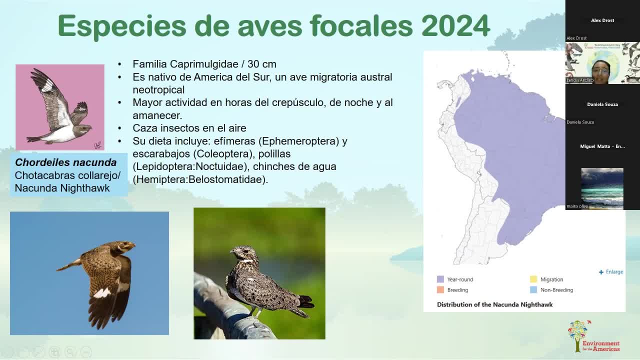 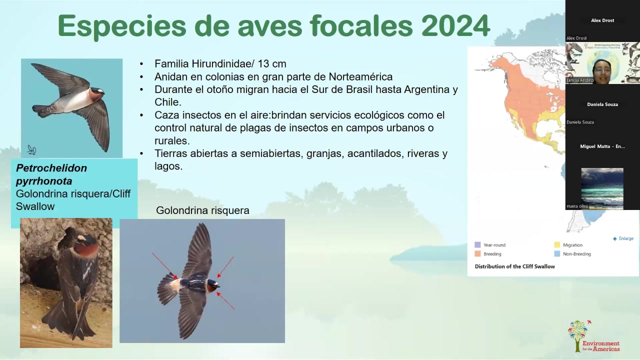 Peru, Brazil, all the way to Argentina. Their diet includes all the different beetle species, The different beetles and moths that we have talked about today, And mainly all of the insects that fly. Our other focal species is the cliff swallow. 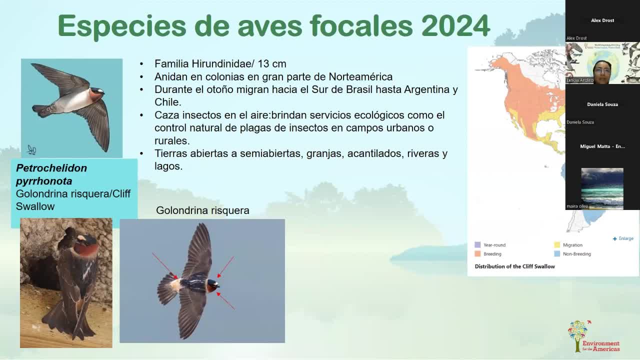 The cliff swallow lives in colonies in great parts of North America. This is a migratory species that flies all the way to Brazil, Argentina and Chile. You can find it in open areas, in semi-open areas, farms along the rivers, along lakes, as well as in cliffs. 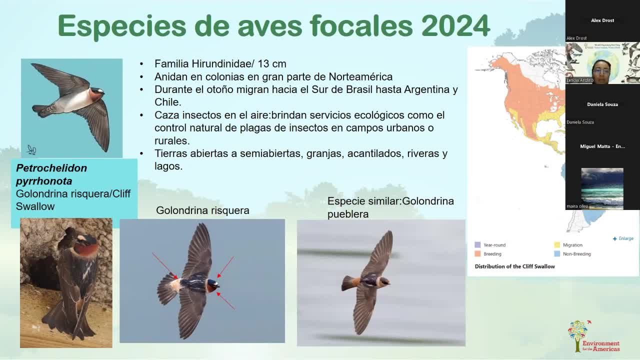 You can see, when we compare here, these species can become particularly confused, Because they can come to a point where they can be very, very different. They can be very, very different. It's coinciding with another species, species which is another sort of swallow that has brighter colors. 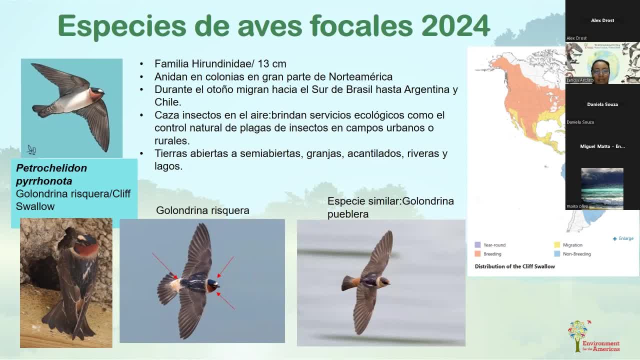 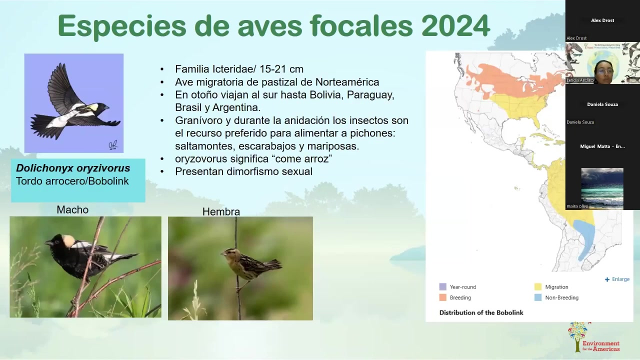 And you can see it in the forehead that they have more of a blue and also a whitish area And the neck is almost like red or brownish red. Those are the difference from the other swallow That is a similar species. You can find it in certain time of the year in the same areas. 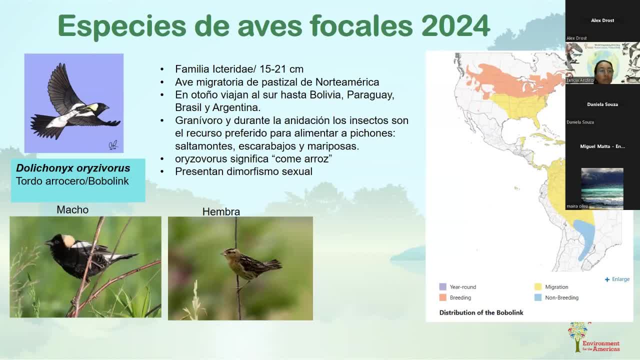 The next that we have is the bobolink, Also common in pastures in North America, But it migrates all the way to the south, to Bolivia, Paraguay, Brazil and Argentina. They feed off grains And they need the insects to precisely feed their chicks during the early stages. 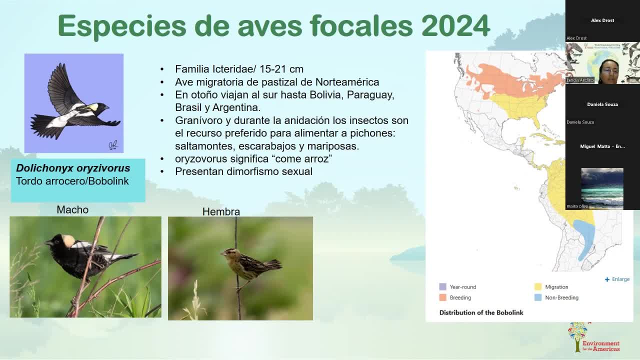 You can find differences between male and female. as you can see in the pictures. The male is a lot darker, almost black. It has a little patch of beige between the head and the forehead And you see some white in the wings, And the female is mostly brown, with some beige areas in the top of the head. 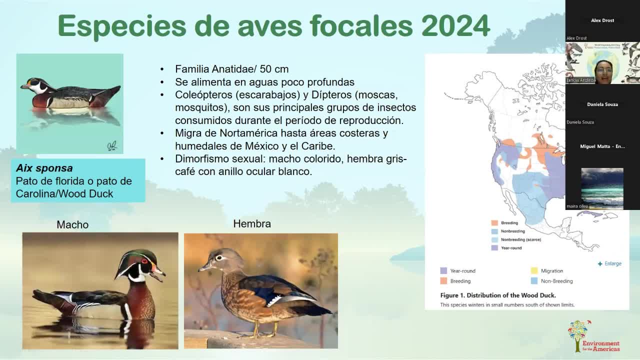 We also have another species, a type of duck called wood duck. It's also called the Florida duck Or Carolina duck. It feeds off shallow waters And you can see it in the distribution map. It can go all the way to Mexico and the Caribbean, mostly in the wetlands and marshes. 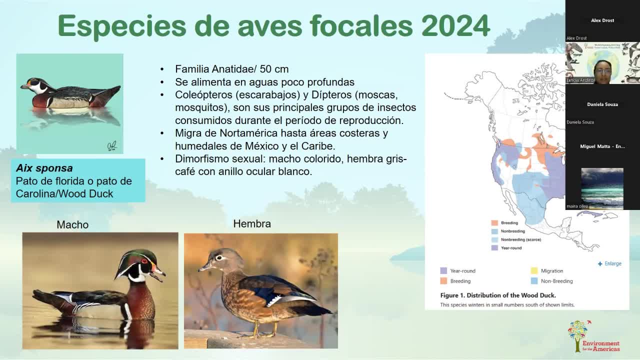 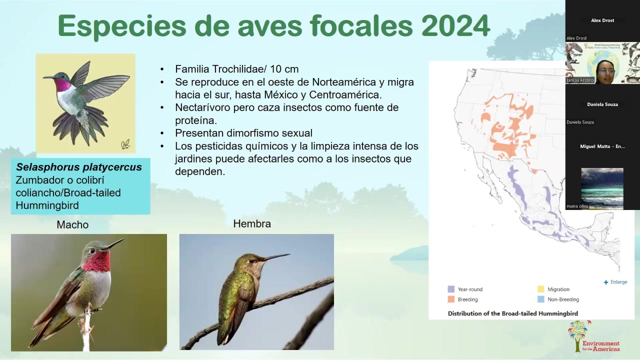 It has a very colorful and it really calls your attention. All the colors that the male presents. The female is a little more discreet in the coloring. They feed off beetles, flies, mosquitoes, mainly during the reproduction stage. We also have another species that is focal for this year. 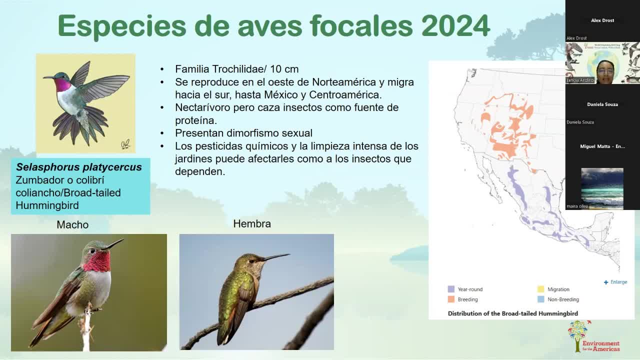 It's the broad-tailed hummingbird. As you can see in the illustration, the tail can become broadened like that. That's why it's called broad-tailed hummingbird. Its origin is North America, but it migrates all the way to Mexico and Central America. 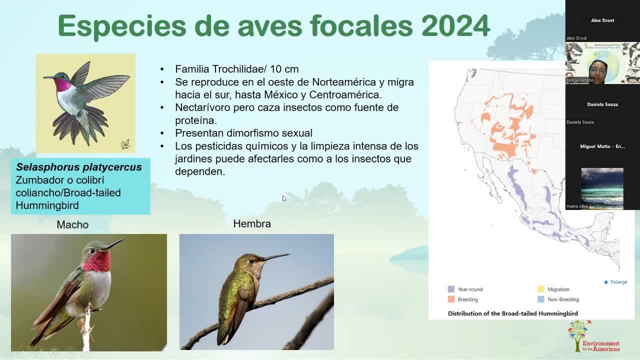 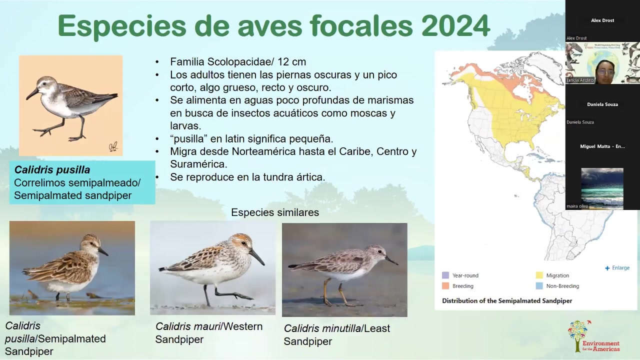 Even though they feed on nectar, they tend to look for insects as a source of protein. The presence of chemical pesticides and the intense cleanliness of gardens could affect them in the way they reproduce and protect themselves. In this same group, we have a beech bird, which is the semi-palmated sand viper from the family of the Scolopacidae. 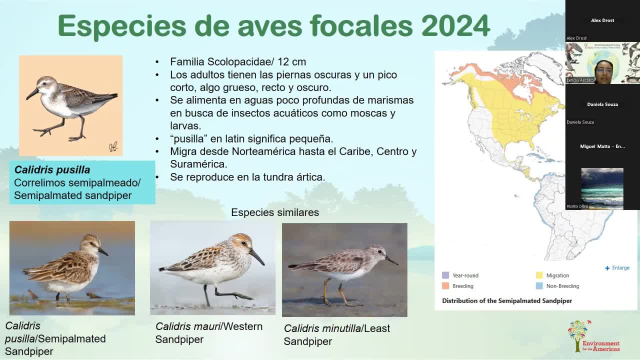 They have a short beak, A little thick. It's sort of lineal and darkened. They feed off shallow waters and of insects that are commonly found in the water, such as flies and larvae. It migrates from North America all the way to the Caribbean, Central and South America. 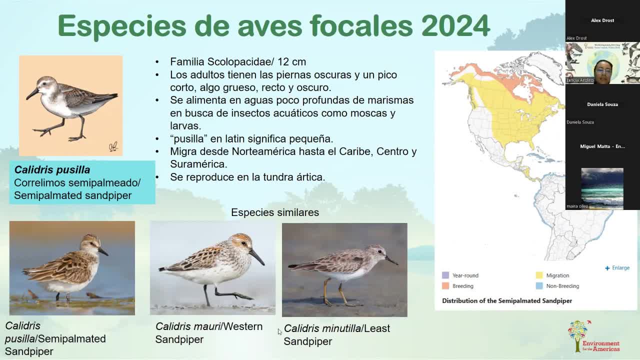 We have other similar species that are common in the tundra. I'm not going to go into a lot of details about these species because our next presenter, our guest, is going to tell us a lot about them. When we're in the field, we can confuse these species. 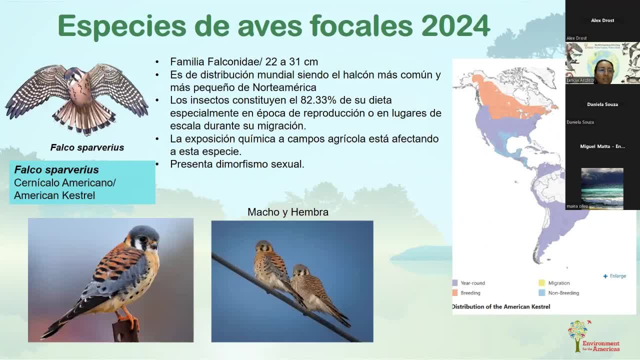 We can confuse them. We can confuse them, But we'll know more about them in a little bit. We have a predator bird from the falconidae family. It's the American kestrel. This is very common to watch in our Central American region. 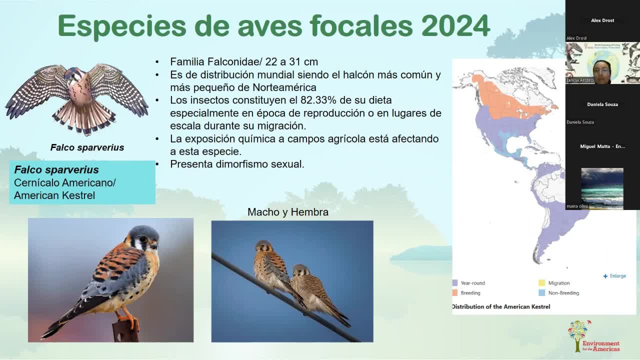 It has a worldwide distribution. It's the most common falcon In the hemisphere. it is the insects that are the main component of their diet. It comes up to 82.33%, especially during their reproductive stage and during the different stops that they make during their migration. 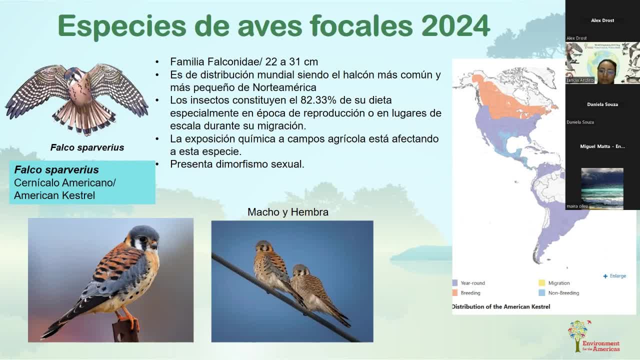 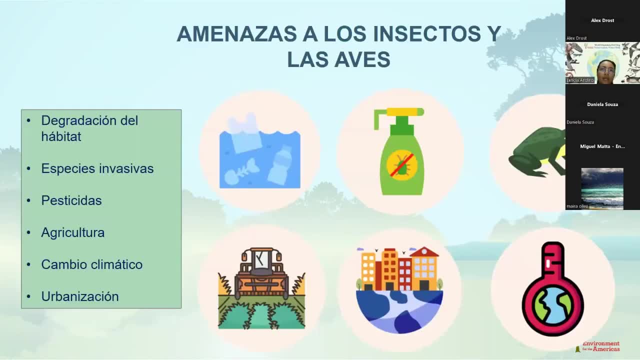 As you can see, the male is a little more colorful And the female has a little more discreet colors. Those were all of our focal species. Now let's talk about the threats. This slide helps us understand the different threats that both insects and birds are facing. 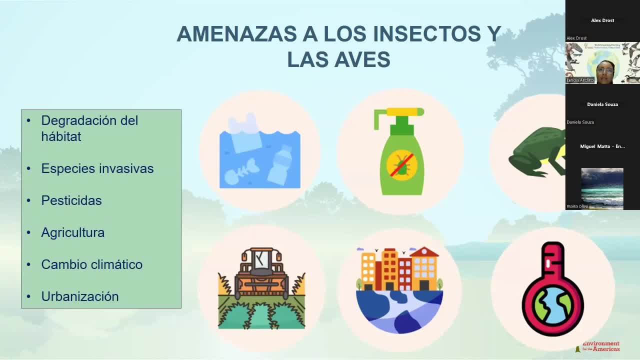 Let's start with the degradation of their habitat and the loss of it. This is one of the main impacts, as well as the use of chemical products for human food crops. Also, the climate change, extreme heat is not something that these species can bear. 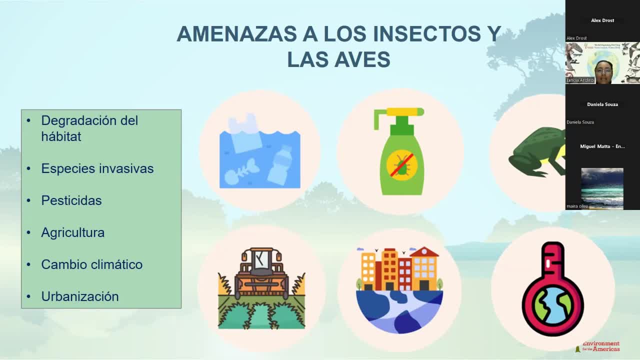 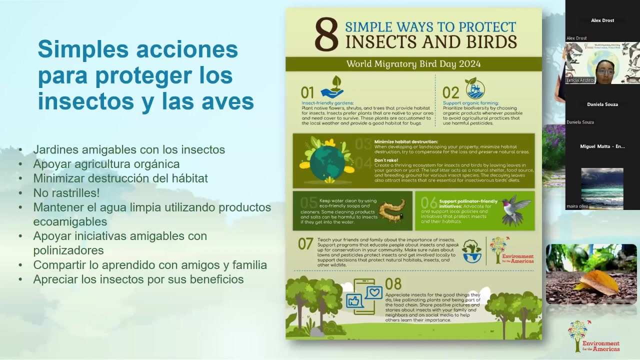 And also some of these species are very vulnerable. They are very vulnerable. They are very vulnerable: The bird species that require insects in their first stages of life. they have decreased in numbers because of the decreased number of insects for food, And one of the simple actions that we could execute in our home, in our community, to protect the insects and the birds is as follows: 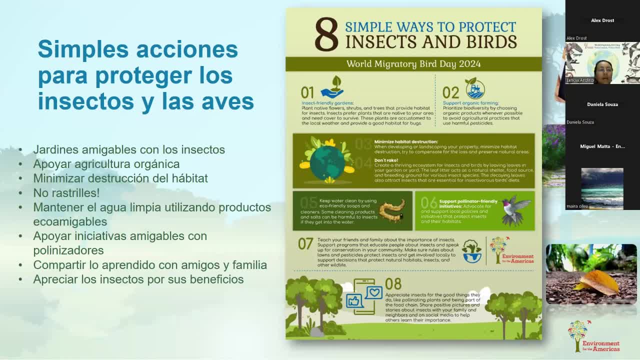 One of them to maintain amicable gardens. This should be one of the main actions for this species because of the harm done to them And this BIOF vibrancy or propriety of the insect is the most common claim. We can snakes抓 Cause they do this. 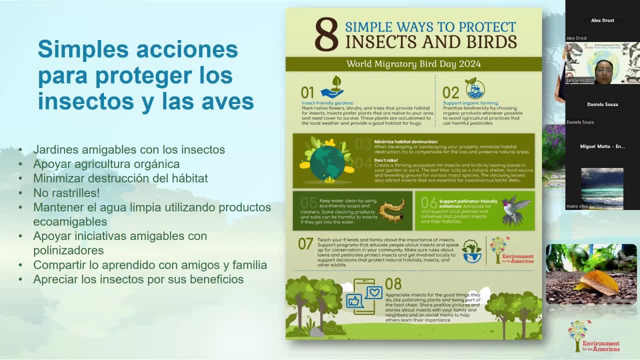 because they are the food of the birds. also, to maintain clean water using eco-friendly products, because if we do not, the products can contaminate the water and affect the birds. also, we need to support amicable initiatives with pollinators. so any policies that are geared towards 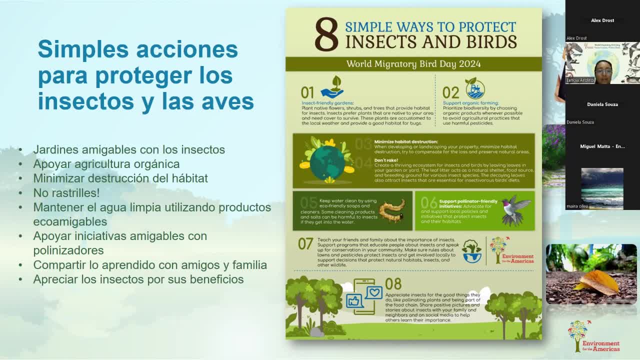 the conservation of habitats for insects and pollinators. also to share everything that you have learned with friends and family, anything that you can learn in these trainings and in other spaces, as well as appreciate the insects for their benefits. some people find them scary, or they may. 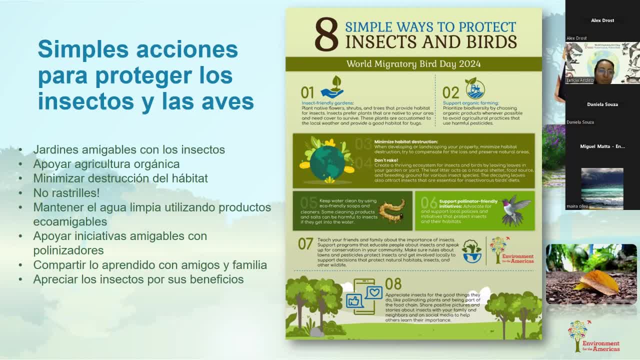 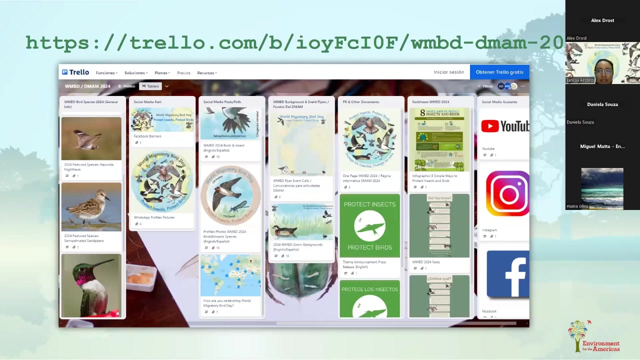 feel they see the group of insects as not something nice. but once we know the different benefits that we have, or that we, the way we benefit as humans, because of their presence, then this can shift our perception. all the information that we just shared- you can find them at this: 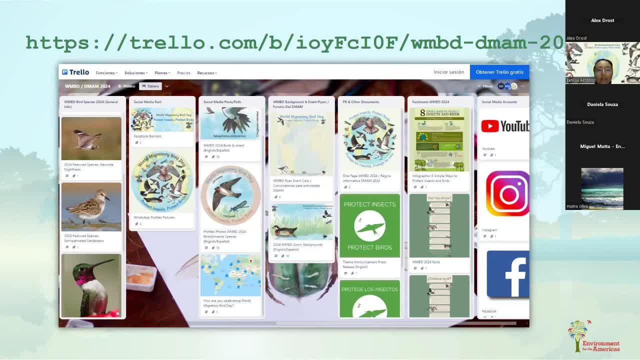 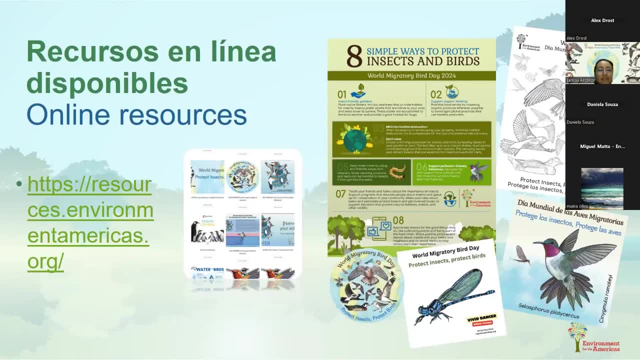 link. it's this platform called trellocom, and there's other actions that you can take to protect these species that we went over. there is also other resources that you can find online on this link and just to remind you that, the second Saturday of May and the second Saturday of October, 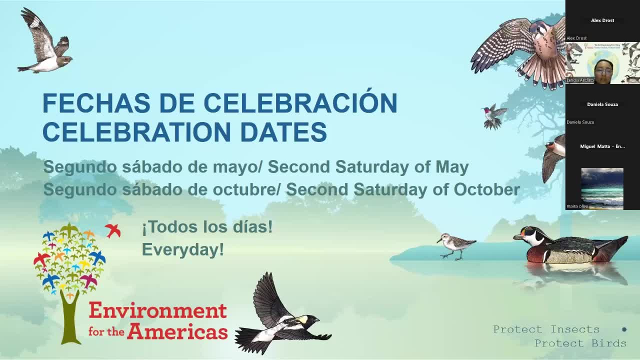 are considered to be the days to celebrate these world days for migratory birds. of course, it can be according to the region and it can vary according to the feasibility within your group. so this is all part of the topics of this year in order for us to become more aware of the needs to 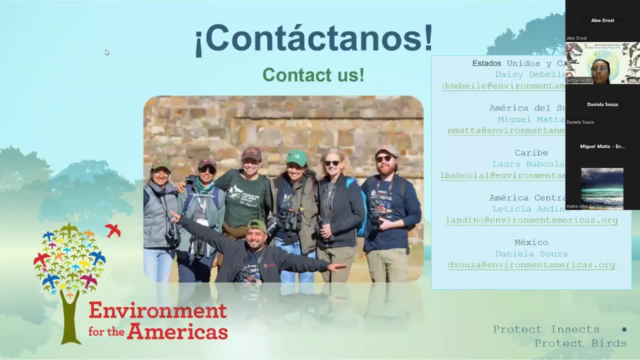 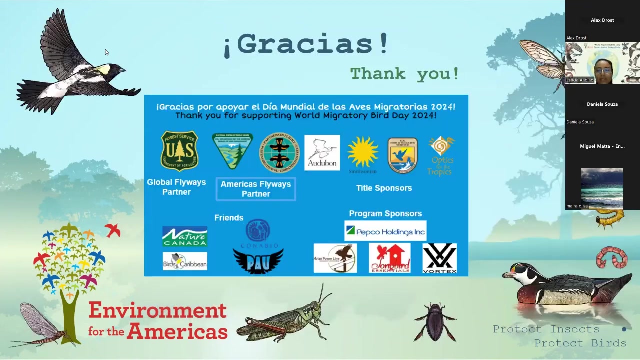 conserve and protect these species. if you need any other information, this is the slide with our contact. we have Daisy the bell in the United States and Canada. we have Miguel Mata in South America, Laura Badula in the Caribbean, Leticia and Dino, which is me, in the Central America region, and Daniela Sosa in Mexico. thank, 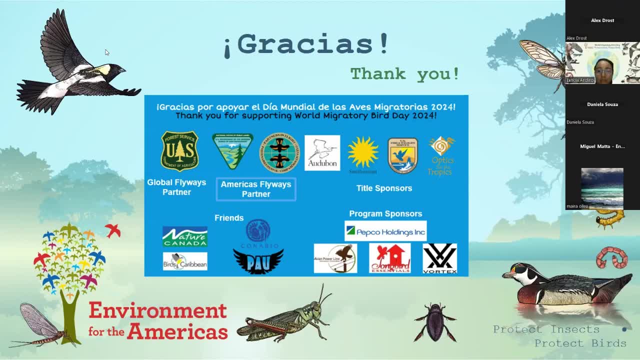 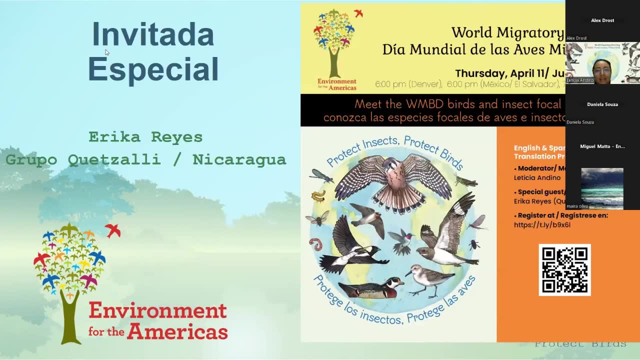 you very much for your attention. you can go ahead and send your calm questions in the chat. right now and at this point we're going to give the mic to our special panelist of today. this is Erica Reyes, from the Quetzali group in Nicaragua. she's going to tell us more about the focus, some of this focal 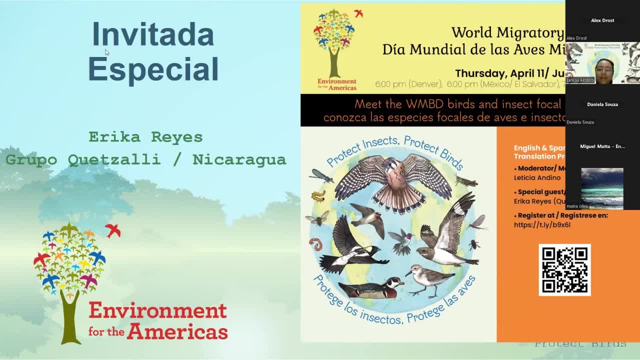 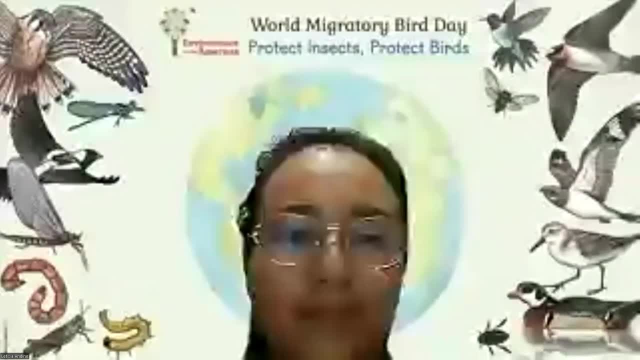 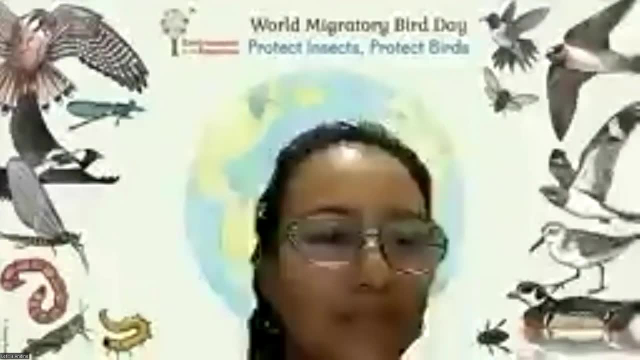 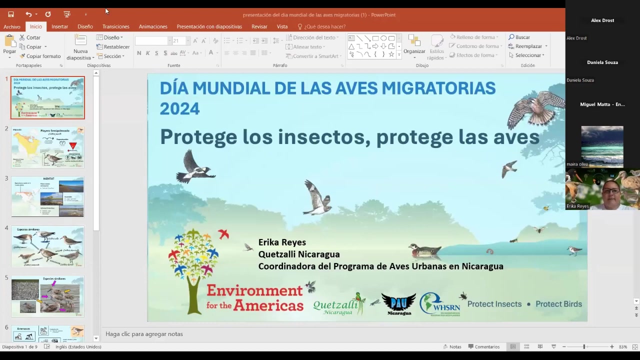 species that we talked about and some of the efforts that they are bringing about in their region for this species. so I am going to stop sharing my screen to give a space to Erica Reyes. go ahead, Erica. good afternoon. can you hear me? yes, we can hear you. all right, and the presentation, if? 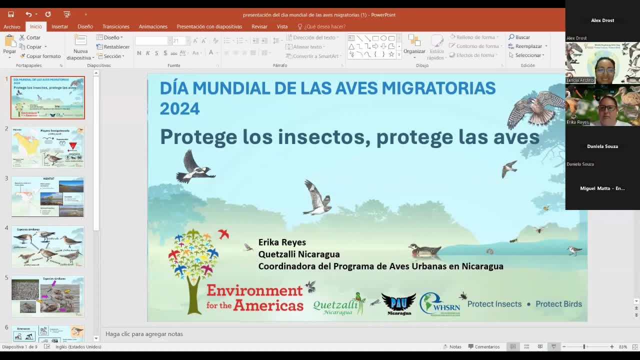 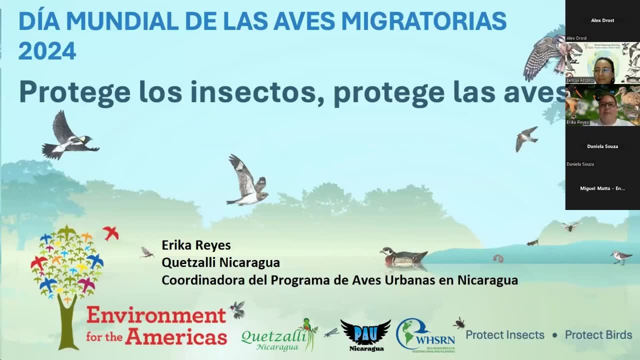 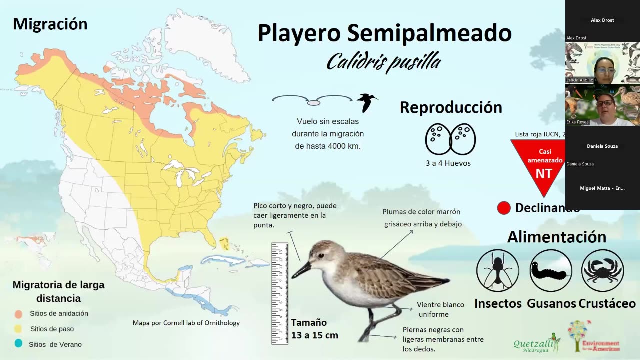 you could please tell me you can see it. yes, we can see it. okay, perfect, good evening. thank you very much for this invitation. it is my turn to talk about the. it's a beach bird, a small one from the. as you can see, the neck is quite short and it's also a small head. 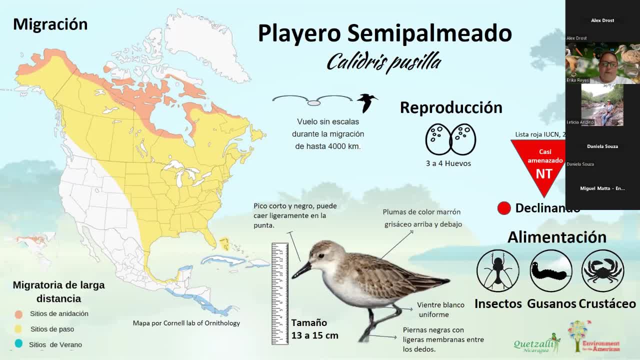 during the reproductive phase. you can see a brownish color in the back or even gray, the abdomen is white and the feet are black. it allows, through a membrane, to maintain themselves standing in the muddy areas and also make sure that they do not sink in those muddy. 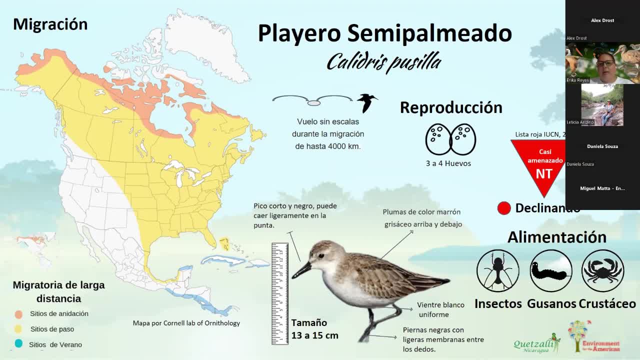 areas and can feed themselves all the way from the base of the peak to the top. it's a rounded Peak. it's not too fine. during the reproductive stage this species will have three to four eggs. during the migration we could go over 4 000 kilometers without resting. they feed of insects. worms, even crustaceans, shellfish and also larvae from a mosquito called the chironomus muscosus, and this species has suffered loss of numbers given a series of different factors, and it is considered threatened because the population is decreasing the size of this species. 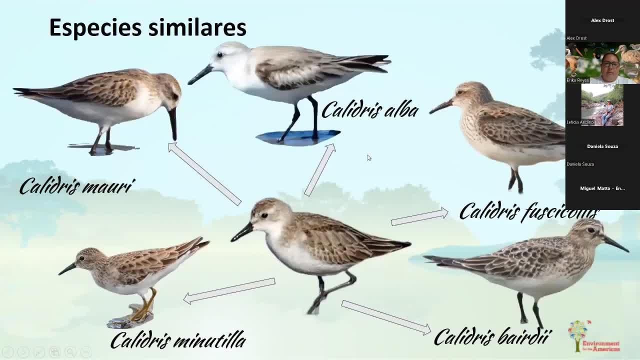 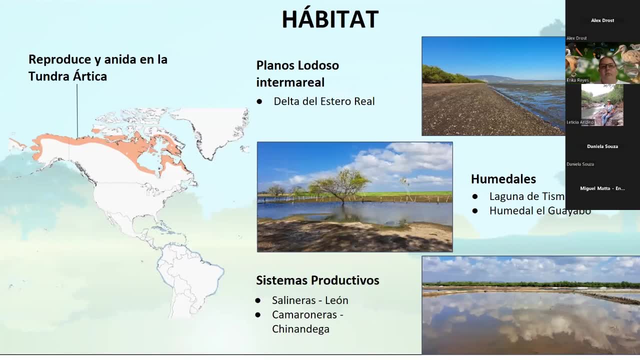 is between 13 to 15 centimeters. the habitat that they tend to visit during the reproductive stage is the chironomus muscosus in the tundra in the arctic, and they also go to the marshes in the stairs estuaries. 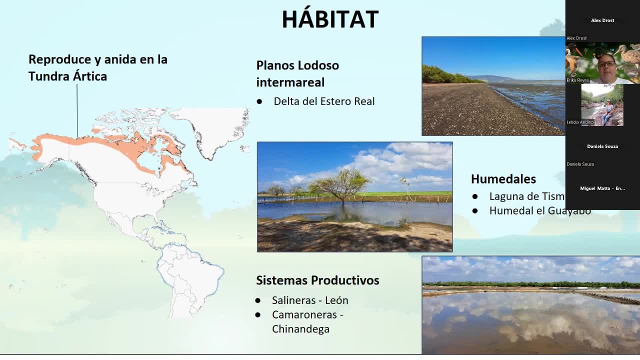 and wetlands, large adult individuals of this species that have been studied is sitio helps them to identify their surroundings. also counts of the, the population of one percent of this species. this species supposes there also has the same and from this place calm, But as a result you can find. 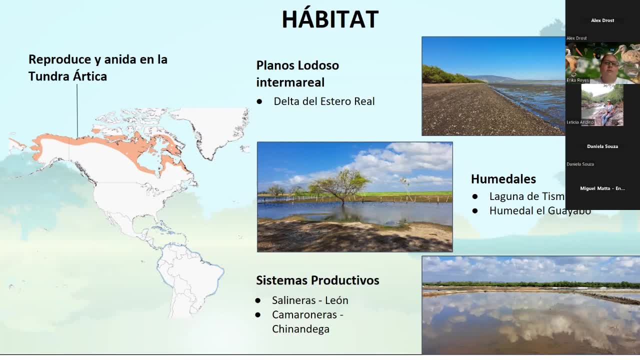 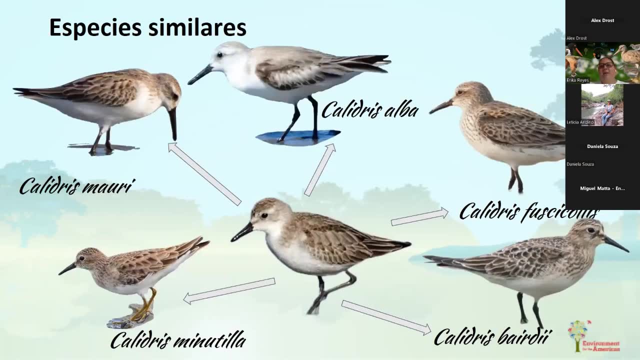 We find them in smaller quantities there. We find it mostly in the coastal areas. Sincerely, beach birds can be a quite challenging group to identify the different species. For example, we have six other species that look very much like our species and 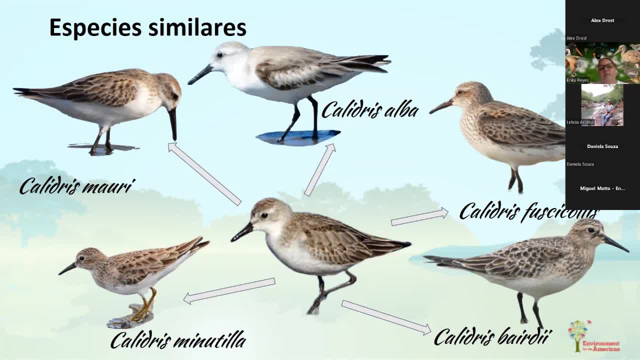 you can see the different similar aspects, But what is the main difference? The Calidris minotilla is smaller and the legs are yellow. The peak is a little longer and finer. With the Calidris maui, this is another species that tends to be confused with the Calidris. 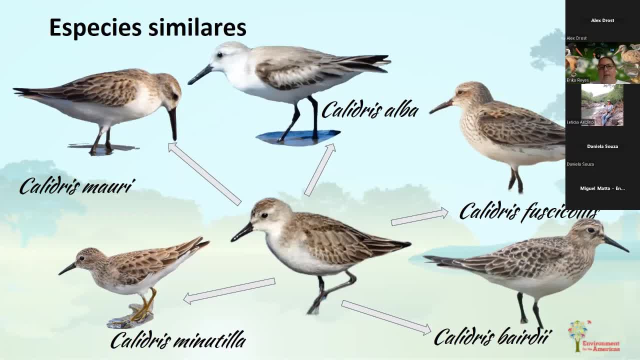 kusila, but the Calidris maui is a little bigger than the kusila. The peak is also much bigger and, as you can see, the base of the peak in the Calidris maui is thicker, but the peak ends up quite fine. They also have 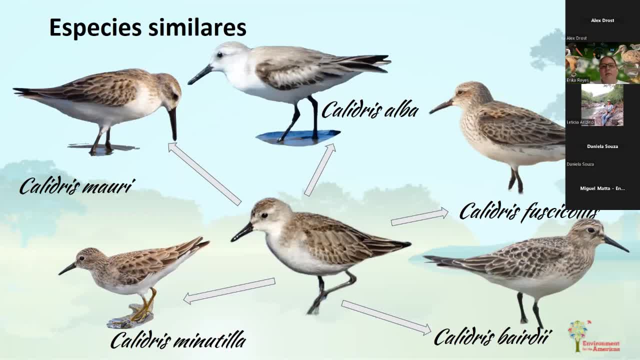 black legs and they tend to be confused with the male, the maui male. It's confused with the Calidris maui. This is the Calidris pusila, which is a species we have as a focal species. Another species that could be confused. 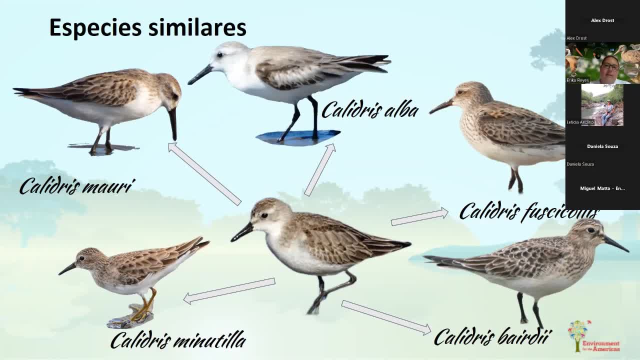 with the pusila is the Calidris alba. The difference with this one is that the Calidris alba is bigger, is whiter and the peak is also black. but it's easier to distinguish because the body is a little wider, heavier. 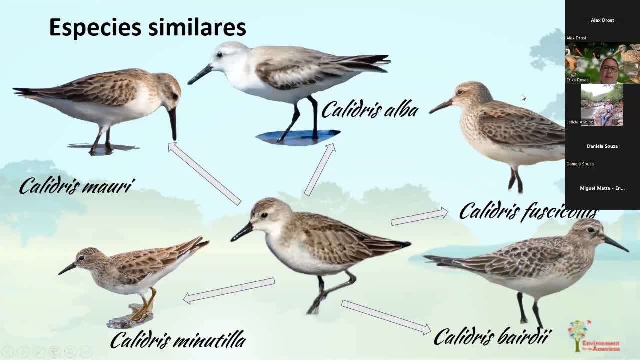 than our species. Another species that tends to be confused with it is the Calidris fusicolis. This Calidris fusicolis is a lot bigger than the fusila and, if you can see in the image, in the chest area it has. 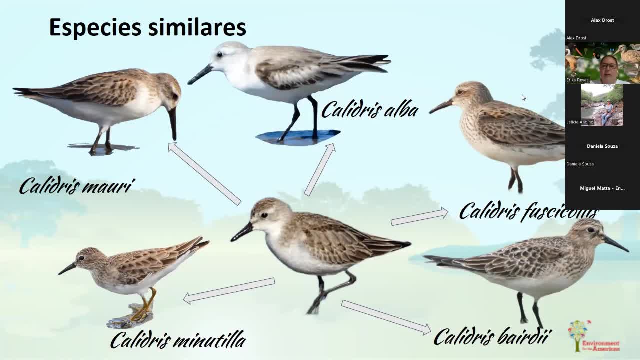 sort of like, some like stripes, and this is something that our species does not have. At the base of the peak it has an orangey color, and the Calidris pusila does not have that. This species also the Calidris pusila. 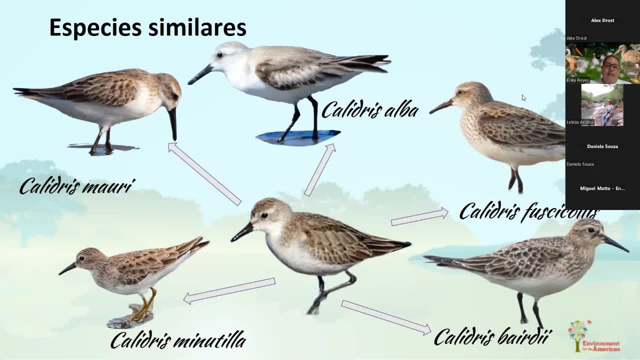 can be confused with the Calidris bairdi. The Calidris bairdi is also a species that is bigger than the Calidris pusila and, if you can see, if you can observe in the image the wings of the bairdi, 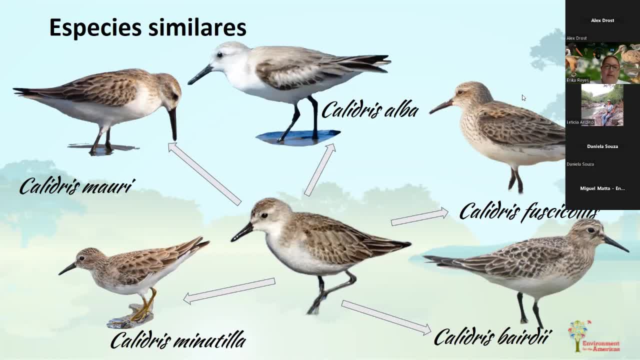 what stands out is that the wing is bigger than the tail, and in the case of the pusila it's not like that. The peak is black as well, but it is a little finer and longer than the Calidris pusila. 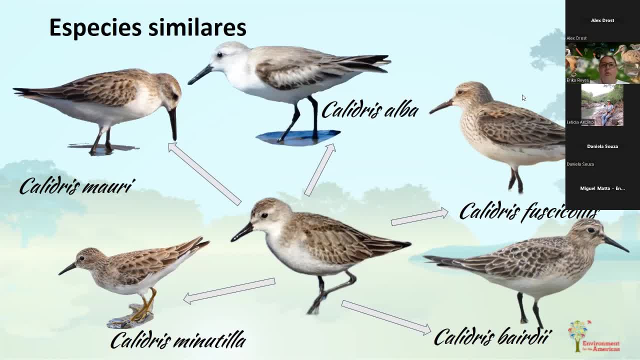 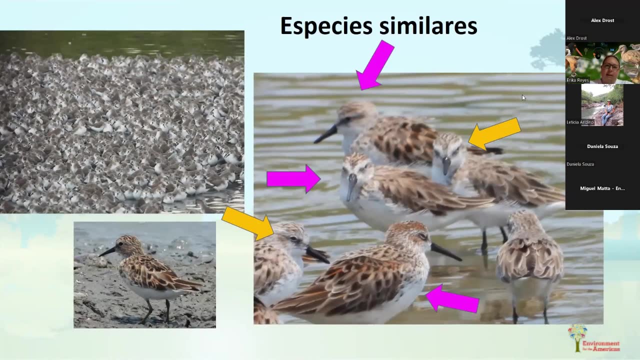 And when you see the big herds of the Calidris, it can be complicated. When you start seeing all these different characteristics, it makes it easier to identify it. Now I would like, if you could please in the chat, tell me. 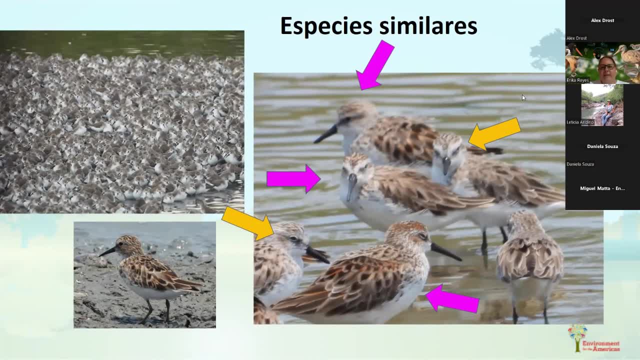 which species you think is the Calidris pusila. I would like to ask you which one is the Calidris pusila, the purple arrow or the orange arrow? You just write the color, the color, the one you think is our species. 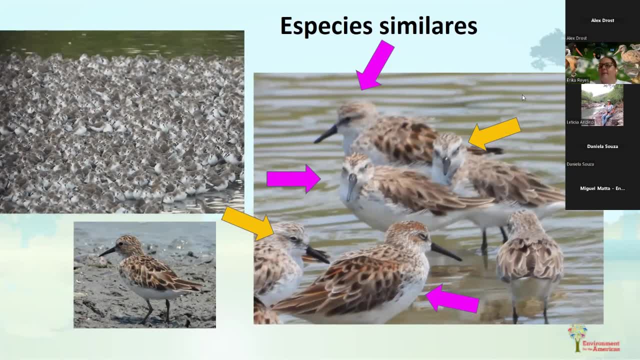 The color, the one you think is our species, And the colors. the colors are all very important Because we see it. It's important to identify, It's important to identify, It's important to identify. However you can identify, if you can see in the image. 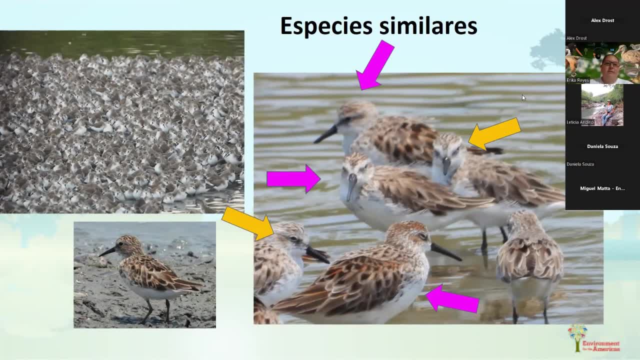 in the left image to the right, I'm sorry, to the left, upper, left. it's very difficult to identify when they're all in great groups like this one in the image And, as I was telling you, according to the characteristics of each of these species. 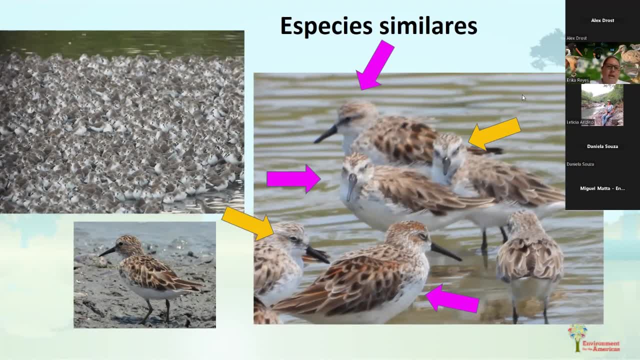 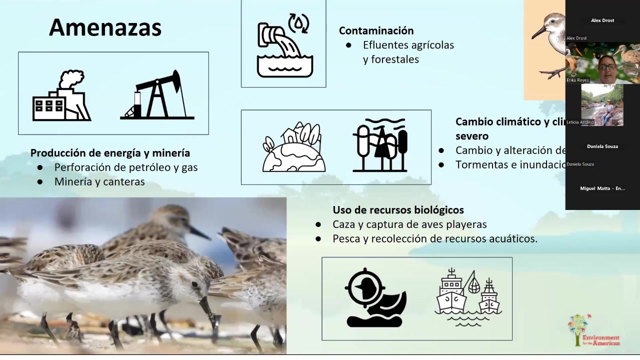 you can identify them as you go. This species I was mentioning earlier is a smaller species than the pocila. The peak is a little longer and thinner. So I would like to see in the chat which one is our calidris pocila. 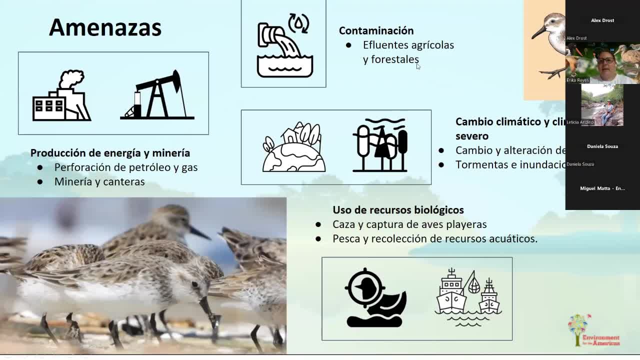 Is it the yellow or the purple? And going again to the threats, as it was. we know that in the case of Nicaragua, given the rain, there's a lot of chemicals being used in the agriculture And all of those chemicals just get taken to the ocean during the big rain season. 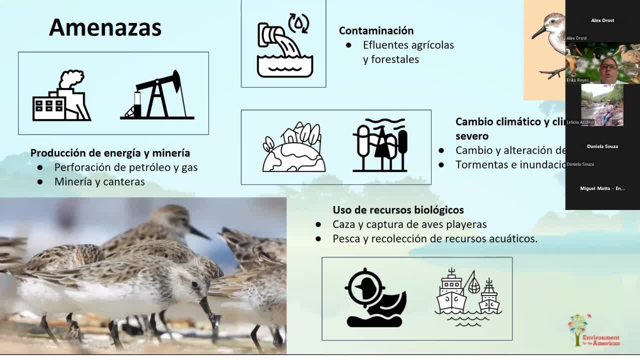 And this can, given the storms and the floods. what happens is that a lot of these migratory species can die along the way through also the alteration of their habitat. Birds are very faithful to space and specific locations, And when they arrive and they find all this pollution. 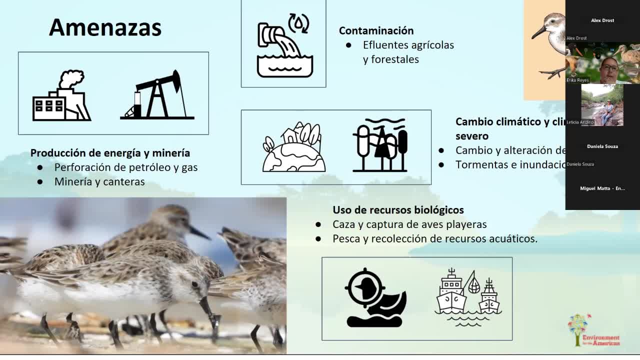 they don't find other places to rest, They don't find places to feed And that is how How calidris pocila has been decreasing in population numbers And also another threat is the use of the biological resources. A lot of these birds can also be hunted, you know. 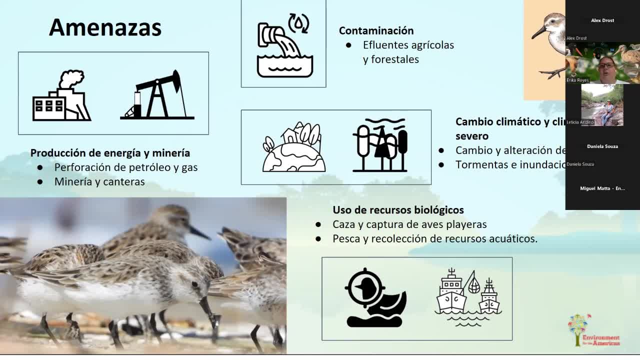 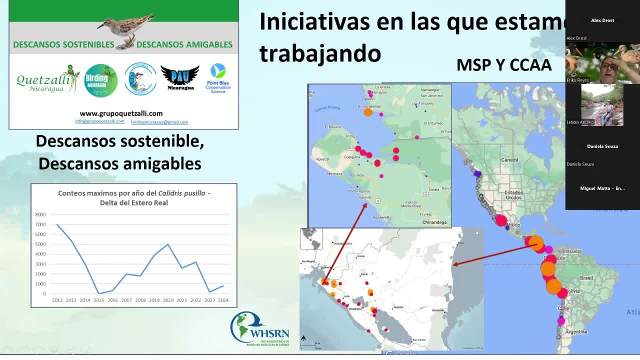 in Nicaragua. in Nicaragua, What we've been doing is a series of work to produce conservation of these beach species, specifically calidris pocila. We've been putting together census for Pacific migratory birds as well as water birds in the Caribbean. 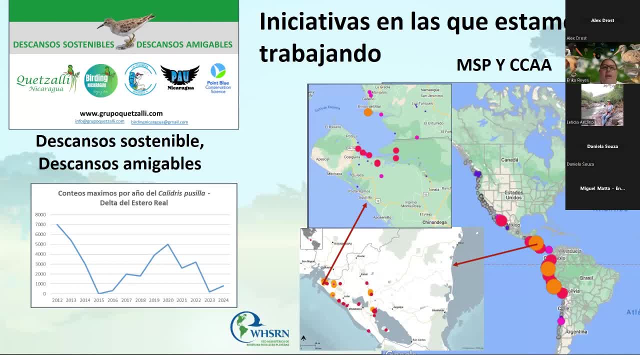 And we've been reviewing different spaces- wetlands, marshes, beaches- and where we've seen the biggest quantity of calidera pusilla has been in the royal estuary in Nicaragua. It's a very important environment on an international level. 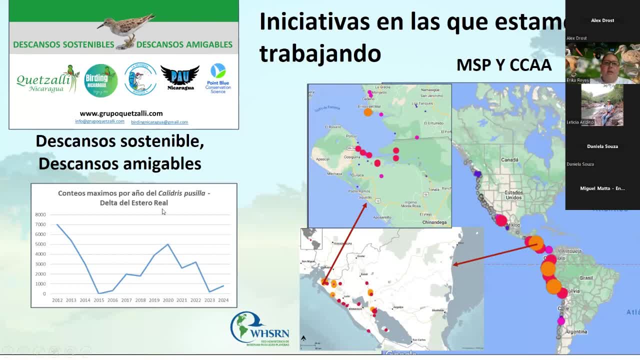 You can find the 1% of these species there And let me show you a graph here: In 2012 to 2024, we can see 2012,. it was counted 7,000 of these individuals And this is how this royal estuary was. 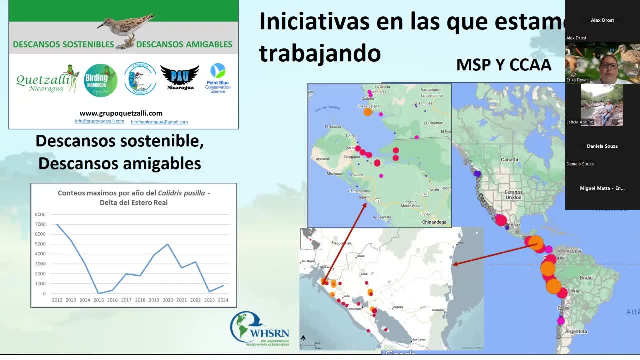 Named an important space for birds, for migratory birds on an international level And also as an amicable space for migratory birds. they've been working in the shrimp farms where we have requested and asked shrimp companies if some of the spaces they don't use in their shrimp farms. 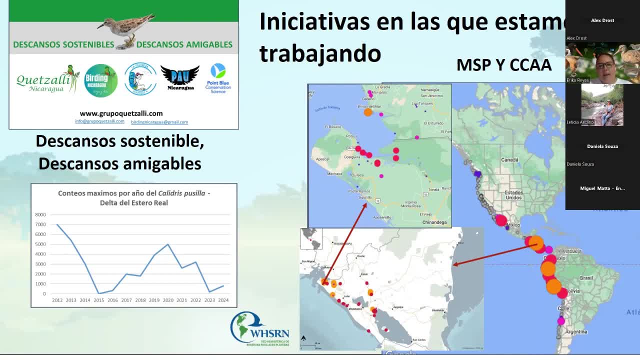 if they could And allow the birds to be there. We have told them how the walls can be amicable for this beach species, Because in previous years we found that when the tide is surging, what we see is that they go to these shrimp farms for refuge. 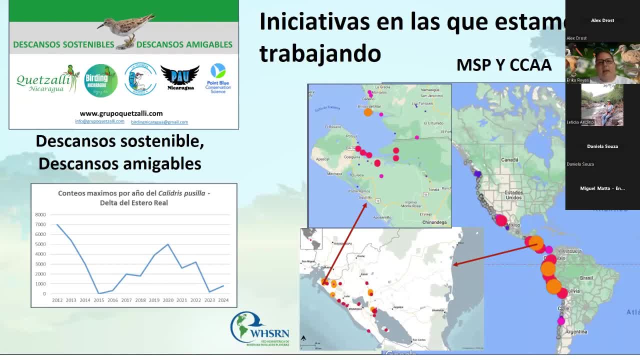 And they use the walls. So what we've been doing is putting together this work of awareness with the shrimp farms and people related to these spaces to make them more amicable spaces for this species to take refuge. We've also reached out to some organizations. 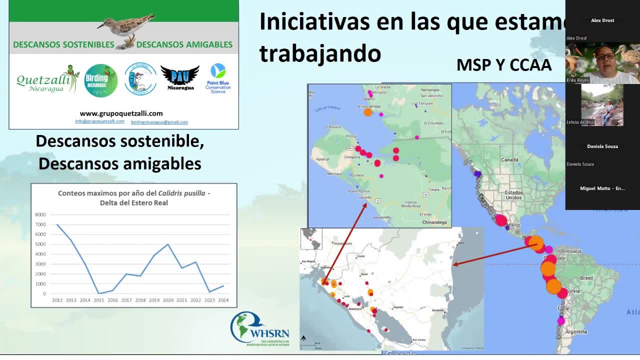 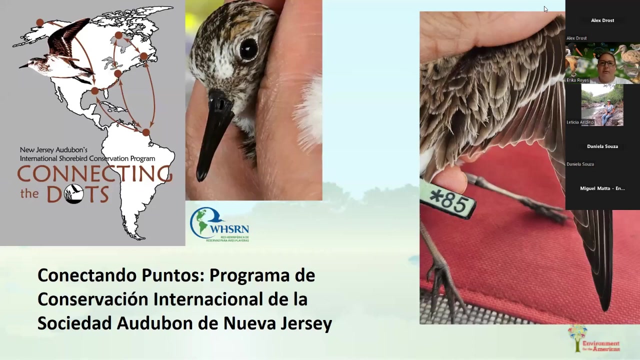 Pond Blue and others- Manamer, for example, Pau, Nicaragua, Verde, Nicaragua- and through them we've been contributing a little bit in the conservation of Calidris pusilla and also other beach species. Another important piece of information that other organizations have: 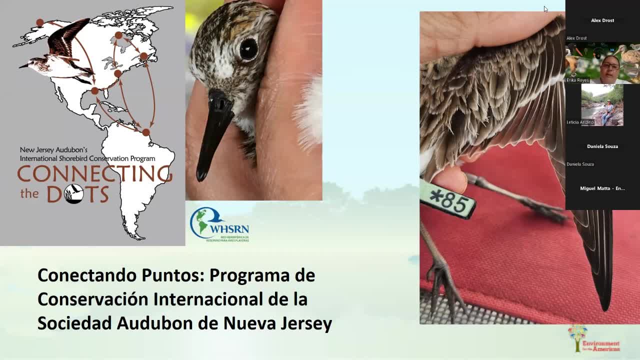 have produced in the conservation. is this international conservation program connecting the dots? This comes from the Audubon Society, New Jersey. The monitoring that they do helps us know the tendency of the population along the natural composition of the spaces. So what they're doing is bring about formation. 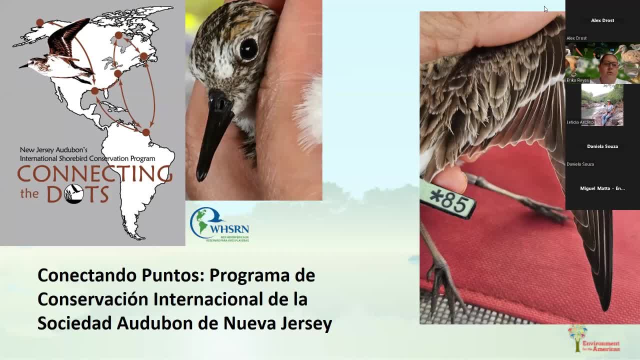 and capacity building of researchers from other parts of the hemisphere for them to participate in this sightseeing campaigns, And also there are other organizations that are involved in this. So what they're doing is bringing about formation and capacity-building of researchers from other parts of the hemisphere for them to participate in this sightseeing campaigns and opening up other areas, and also to bring about the 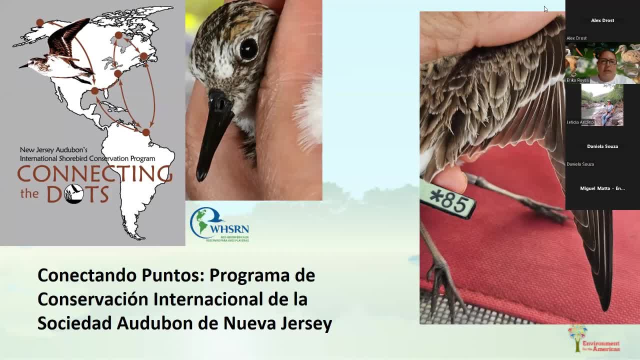 us as quetzali, we've had the opportunity to participate, salvador morales. they have had the opportunity to travel all the way to delaware, which is another important space for this species, because they there is where they feed off the crustacean species, specifically a type of crab from the wetlands of delaware, and it helps this species and the 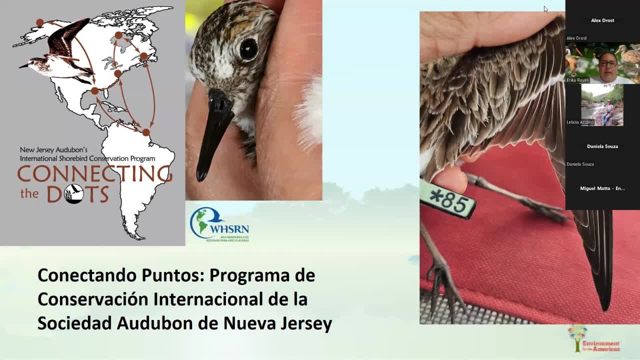 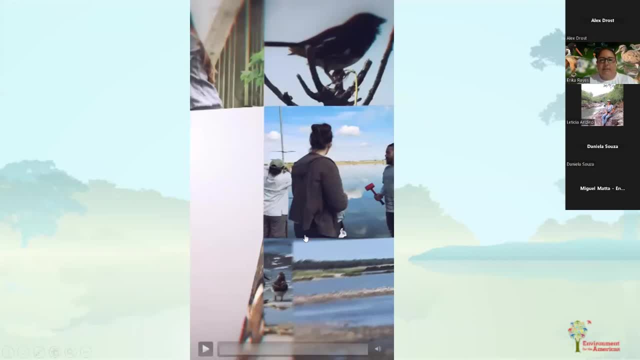 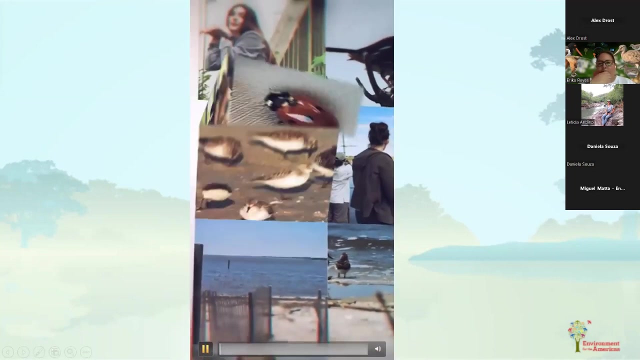 different studies that they produce along the time, for these are studies that they are conducted for years and allow them to realize the behavior of the population. and lastly, i have this video. let me know if you can actually hear what this video is saying and again thanking manomet for the opportunity that has given us to realize a series of studies here. 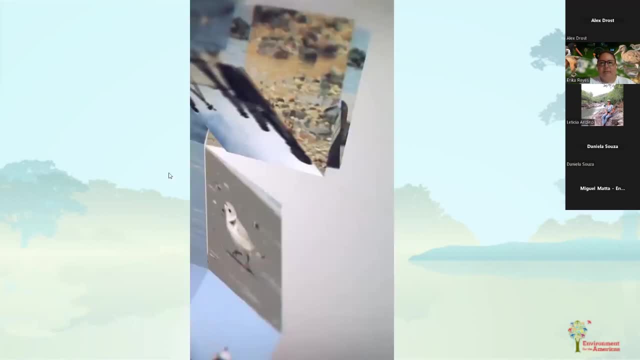 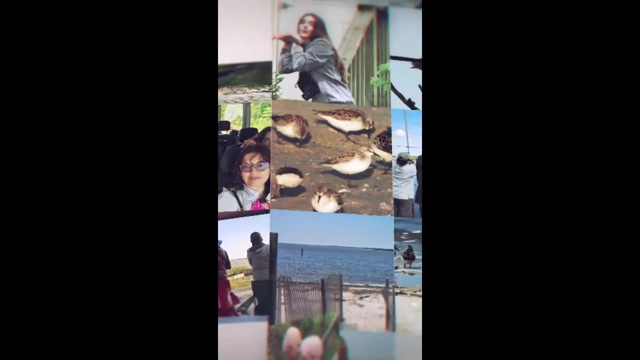 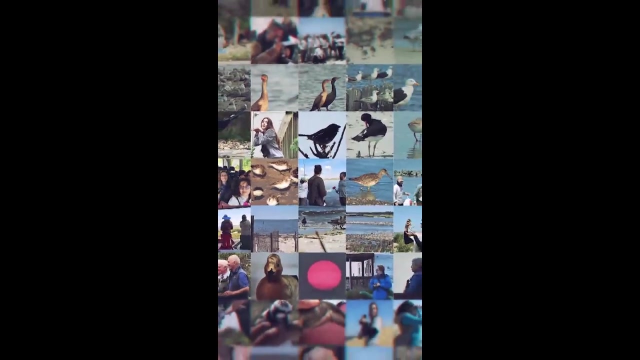 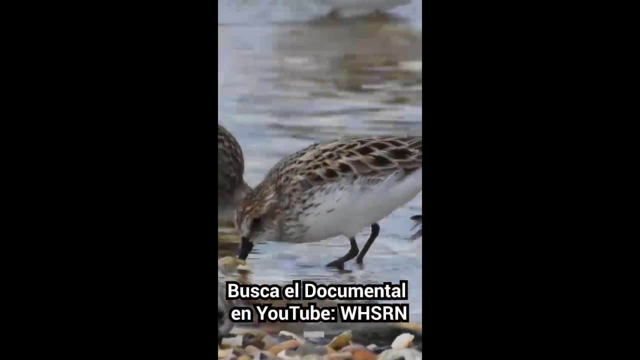 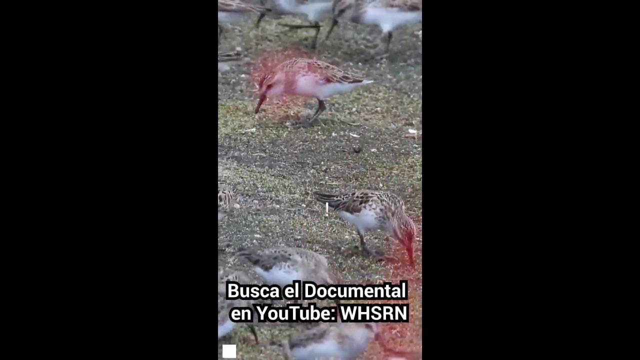 in the delta of the estuary, the royal estuary in nicaragua, the know, one of the stop sites of the semi-palmed heron, and how we connect several partners from Chile, Argentina, Brazil, Nicaragua, Mexico and United States to monitor and protect. 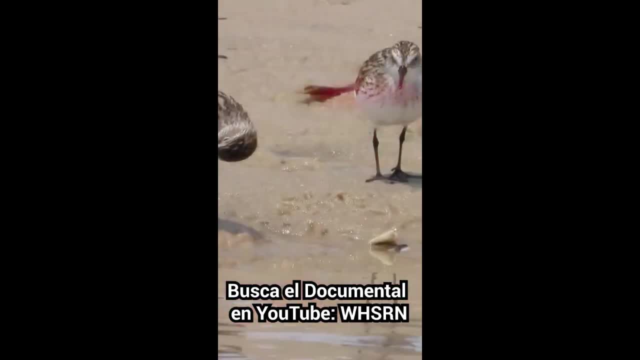 to the s. They are Hospitality throughout their life cycle. the semi-palmed heron is a migratoria que nos conecta. Es urgente que sus hábitats en América del Sur Centro y en México sean protegidos. 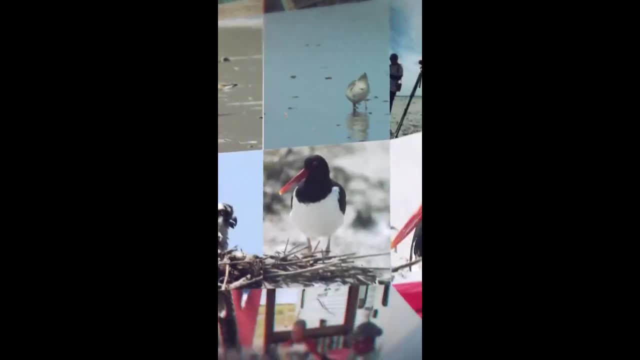 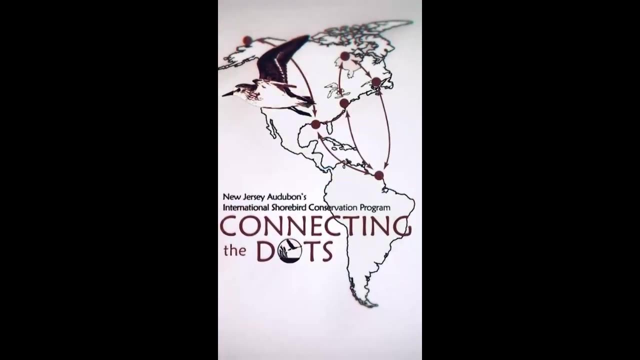 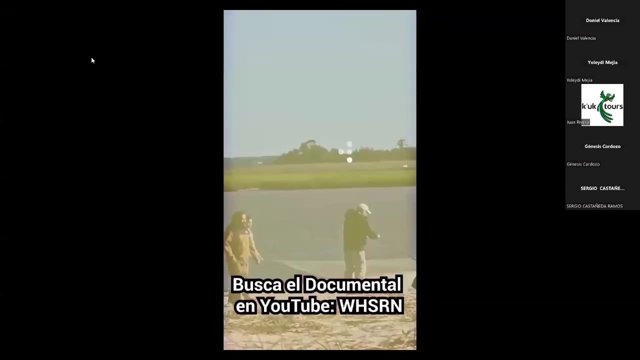 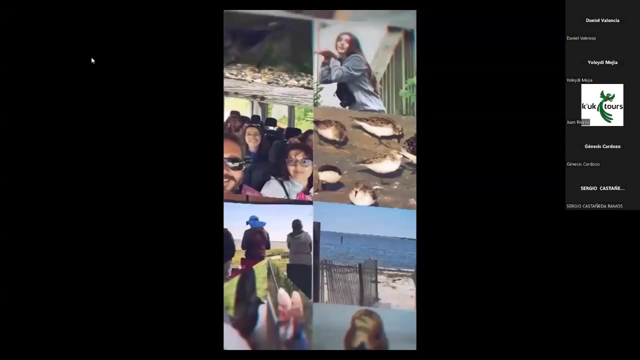 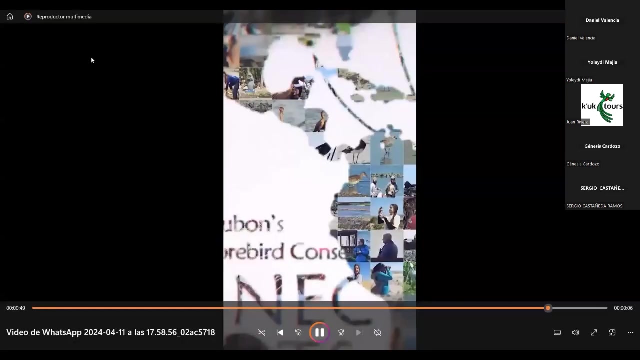 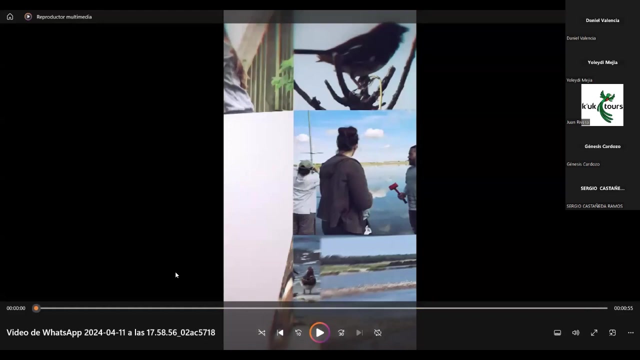 Well, this video was about the experiences that have been lived by many researchers in Delaware When they are birdwatching this particular species, especially when they're feeding on the type of crab that they're so commonly feeding seasonally in Delaware. again, I want to thank Environment for the Americas. 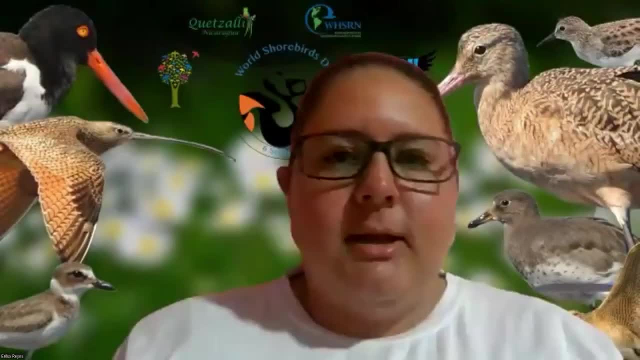 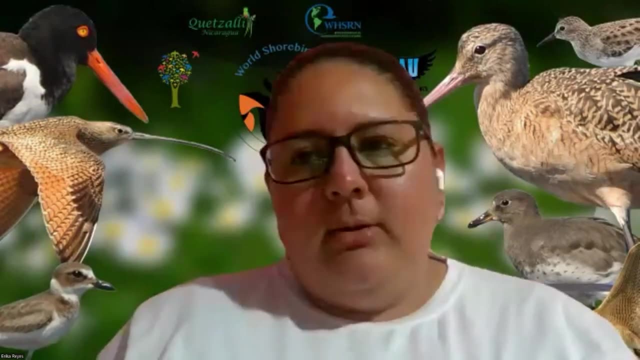 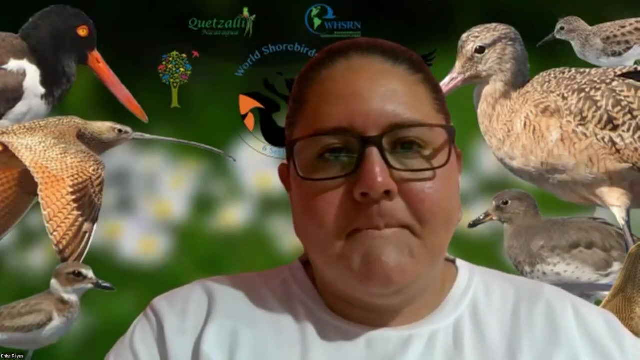 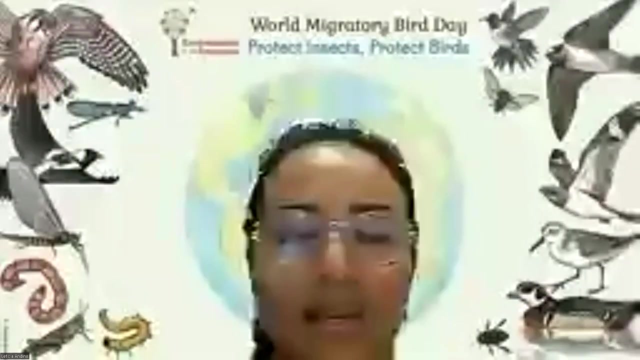 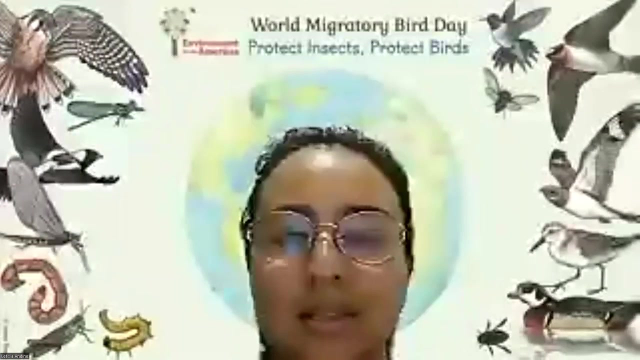 for this opportunity and to be able to present some of the information that we're doing here in Quetzalini Garagua. Thank you, Thank you very much, Erika, for the presentation. All the efforts that you're putting together are so interesting in Nicaragua and in that. 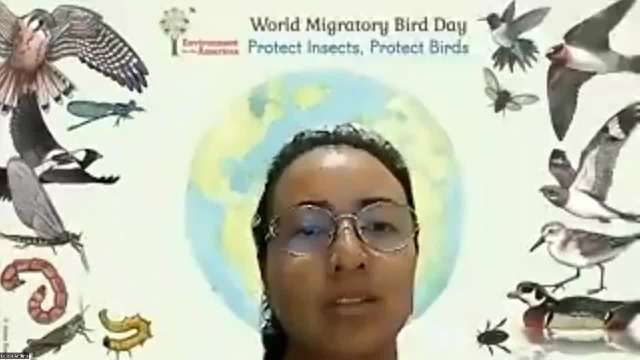 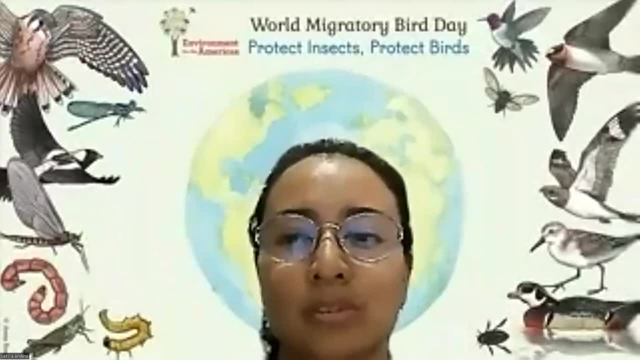 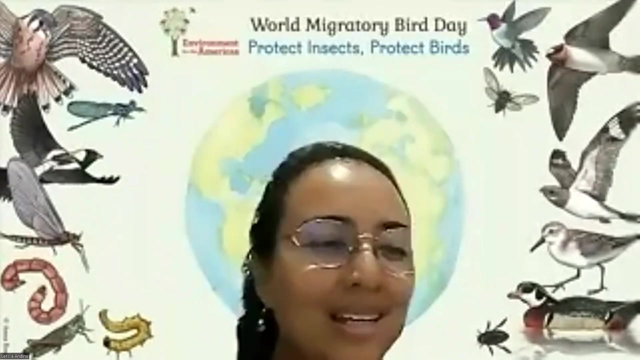 area where you've been able to register. this species, as we're seeing, is one of the species that its population is decreasing And that is why we're putting it as a focal species in our efforts of conservation. And also very important and interesting the way you can compare it to other bee species. 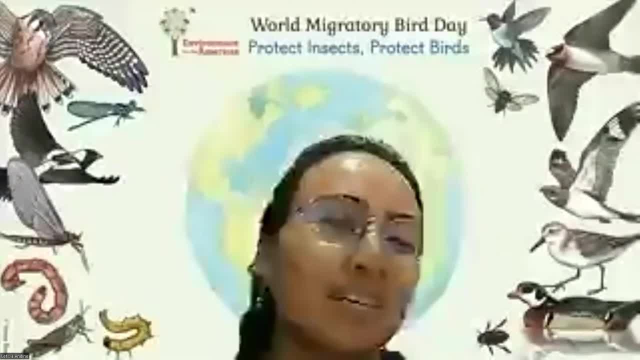 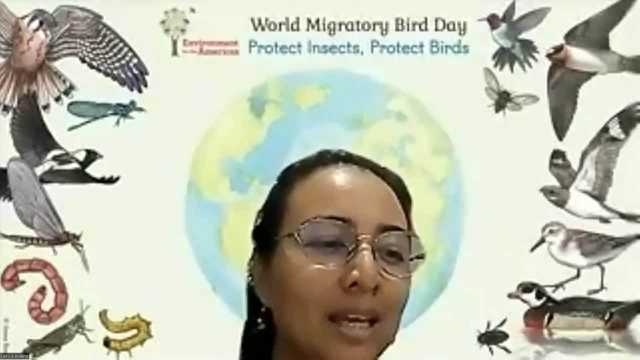 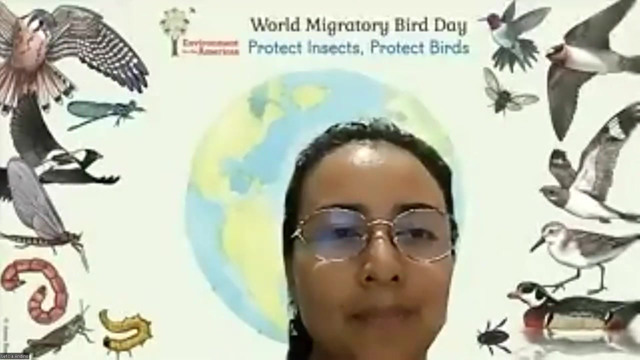 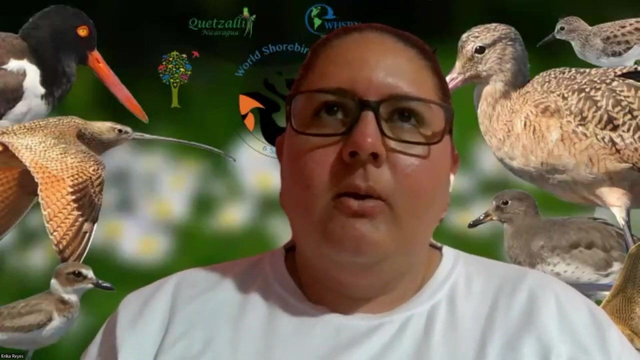 Important to know the different aspects that help us identify species, because this is the way The data, the records, the data, the data is important. registration that you hold, the documentation of the data, can come about. It depends on that identification. So have you been able to see any banded or ringed birds?